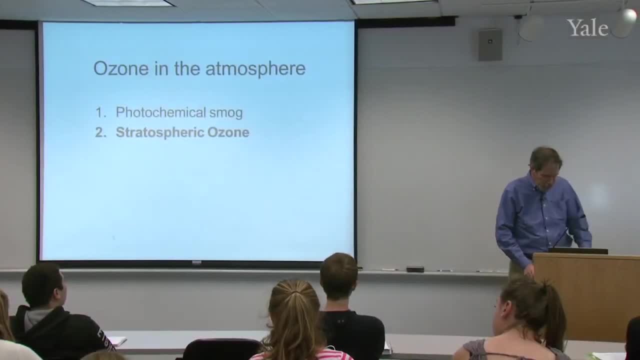 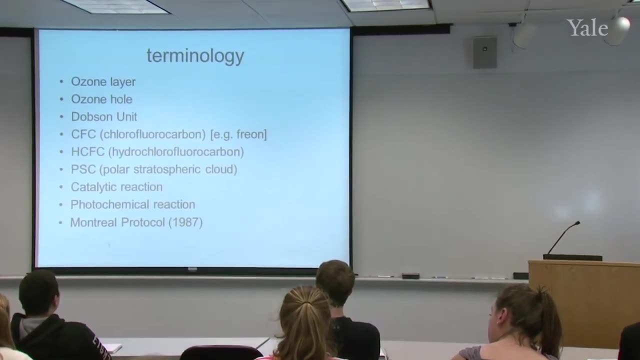 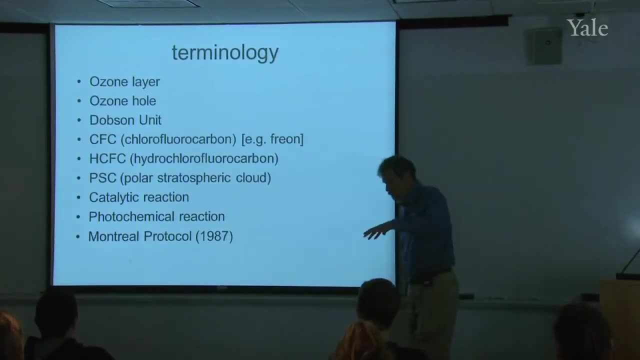 OK, so we're going to do the stratospheric ozone problem today, and these are the new terminology that you should be aware of. So we'll talk about the ozone layer and then the ozone hole, The Dobson unit I'll discuss, I'll define as a measure of 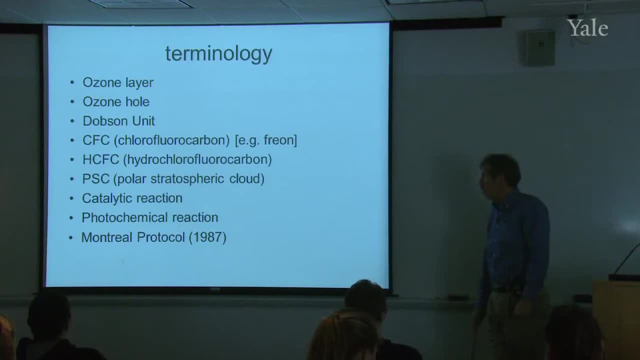 column integrated ozone concentration. We'll be talking about CFCs, which had been used as the primary liquid in refrigerators, And you need to have a fluid that flows back and forth between the cold sink and the warm sink in a refrigerator, And CFCs was the common chemical to do that. 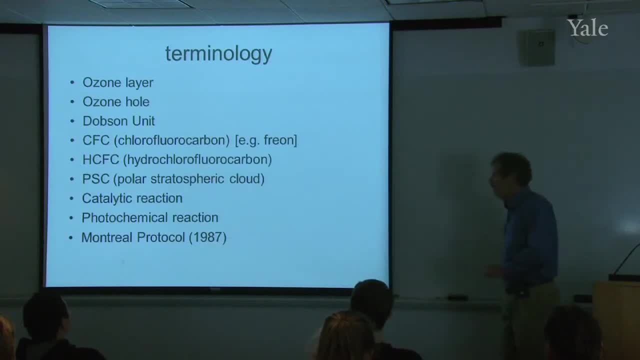 But now they've been replaced largely by HCFCs. the hydrofluorochloroplast Hydrochlorofluorocarbons say that 10 times fast, And so I'll define those as well. We'll talk at some point today about polar stratospheric. 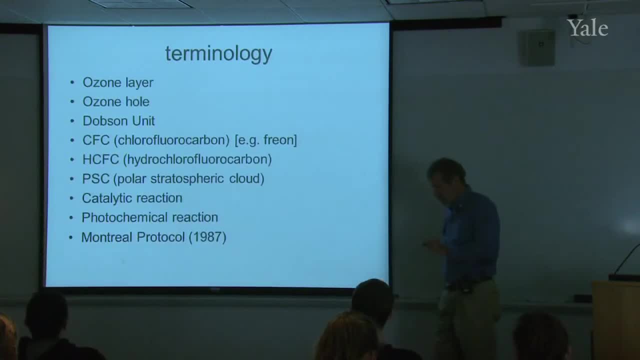 clouds. catalytic reactions, which are reactions in which one particular chemical compound allows the reaction to go forward but in the end itself isn't changed, So it can be reused over and over again to make the same chemical cycle go forward. Photochemical reactions, which are chemical reactions that 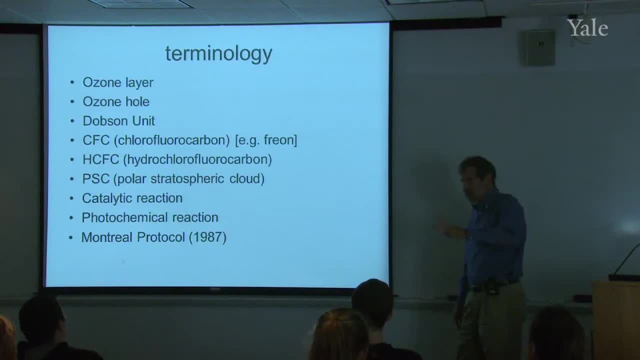 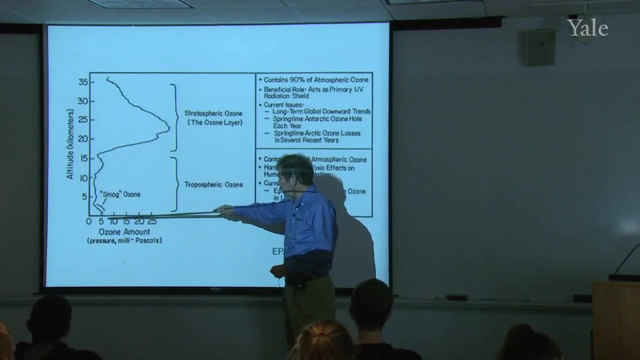 involve light. You have to have photons of light in order for that reaction to go forward, And we'll talk about the Montreal Protocol. So all this will come in turn today. First of all, so I showed this diagram last time as we discussed this part of the ozone issue. 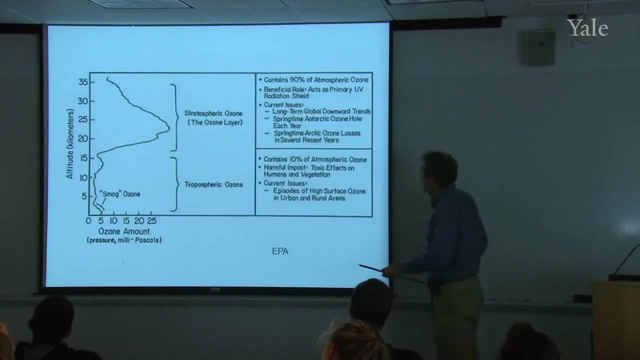 But now we're going to talk about the ozone layer And, as it says here, contains 90% of the atmospheric ozone. So if you do a column integration, you're going to have a column integration from the top of the atmosphere to the bottom. 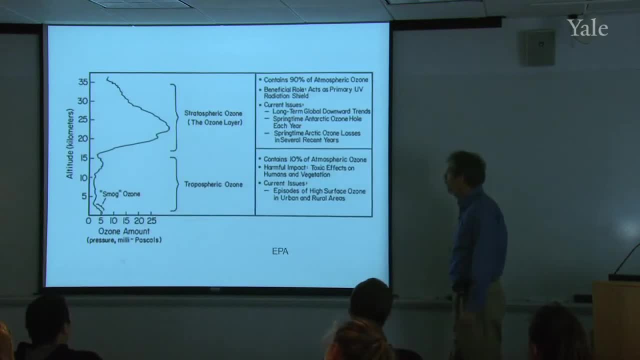 Most of the contribution comes from the ozone layer. What's plotted here is the partial pressure of ozone in millipascals. Remember that the total pressure, the air pressure, decreases strongly and exponentially all the way on up through the troposphere and the stratosphere. 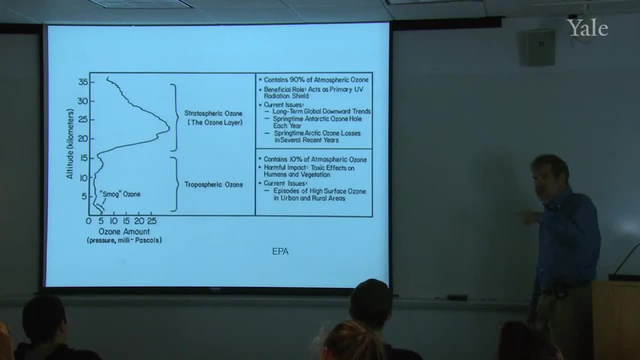 So this has a very different vertical structure than the total air pressure. It has a beneficial role. It acts as a shield against ultraviolet radiation that would otherwise cause skin cancer, skin damage, And the current trends are a long-term global downtrend in. 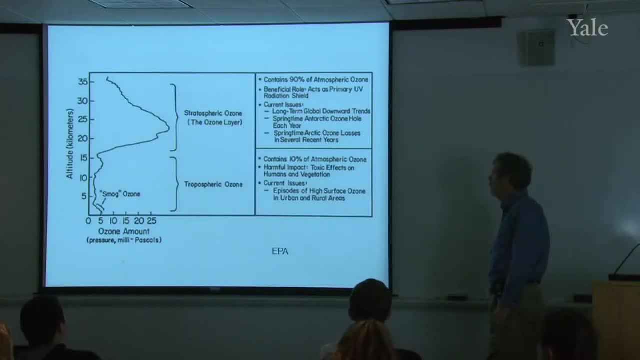 stratospheric ozone And then, most famously, the ozone layer is going to be a result of this ozone hole, which occurs in the springtime of the Antarctic part of the Earth each year, And then some more recent discussion about possibly this starting up in the northern hemisphere as well. but this is 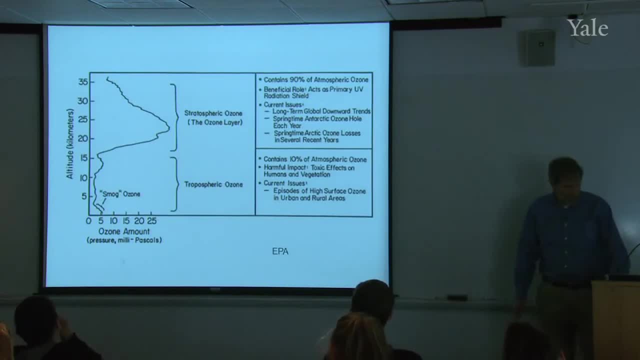 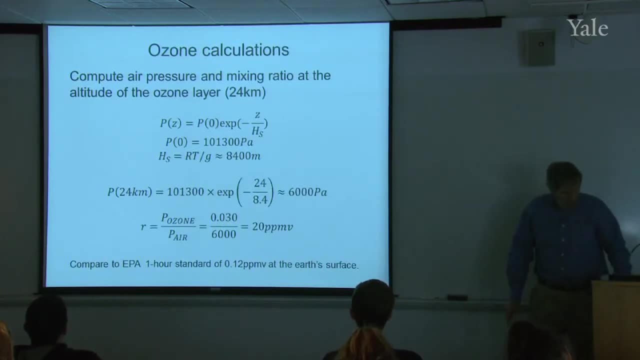 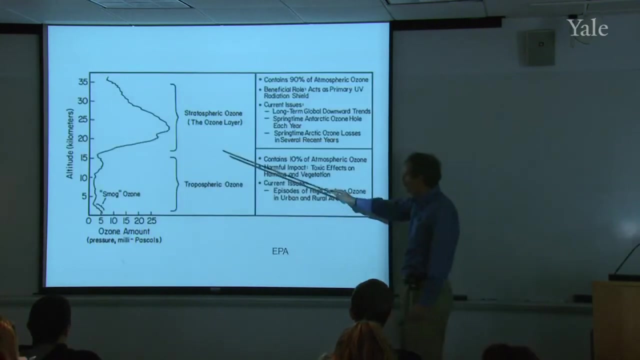 not as well documented. So just a couple of calculations then. So I want to compute the mixing ratio. I'm going to use a PPMV for ozone to air using this point on this slide, So I'm going to say that, that at about 24 kilometers altitude. 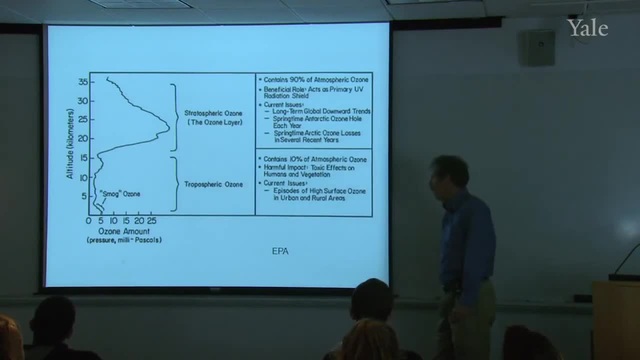 you've got a partial pressure of ozone that's about 30 millipascals And I want to convert that to a mixing ratio because that's what we've been used to using what we used last time. So first of all, I'm going to use a mixing ratio. 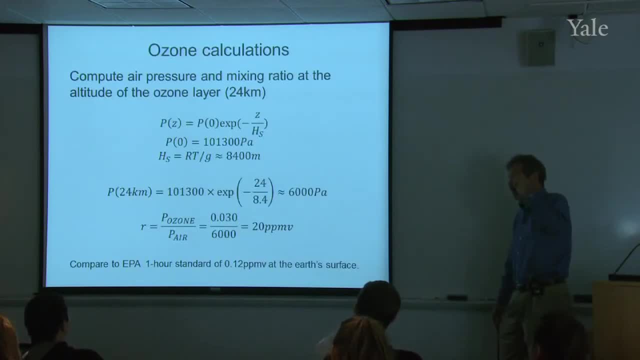 Well, because it's going to be a mixing ratio, I need to know how much air is up there as well, Not just how much ozone, but how much air. So I'm going to use this simple formula that we've used quite often in the course. 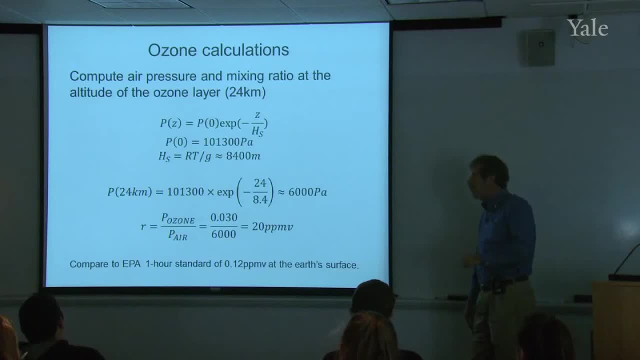 It's the approximate exponential form for pressure as a function of altitude. where you use a scale height h sub s, you know the pressure at the surface of the Earth, you know the altitude you're inquiring about and this will give you the pressure. 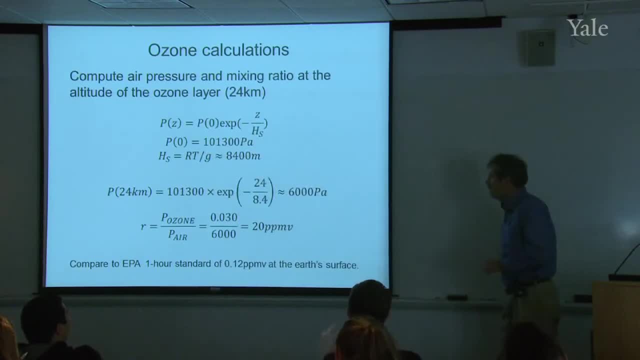 The pressure at that altitude, So sea level pressure, will take to be 1,013 millibars, which is the standard average value. Convert that to pascals. The scale height, as you recall, is RT over g, which is: 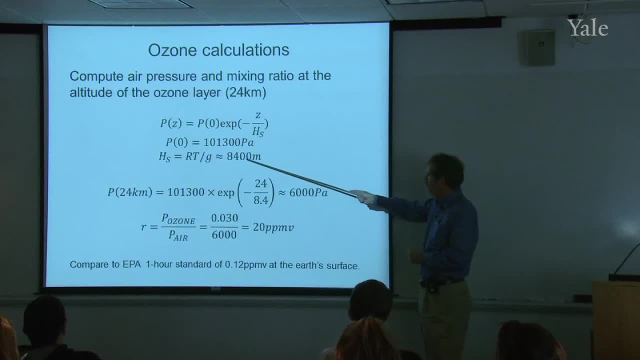 about 8,400 meters for the Earth, the Earth's atmosphere. So I'll put 24 kilometers up here, that scale height there, and I'll put the sea level pressure there, And that's this formula here. So I put everything where I said. 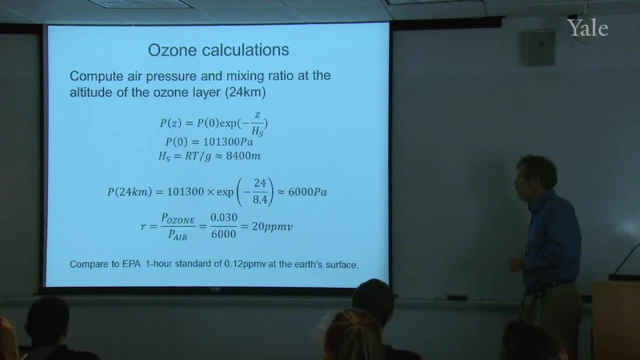 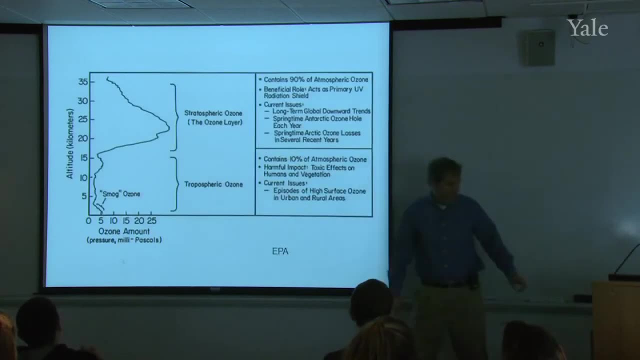 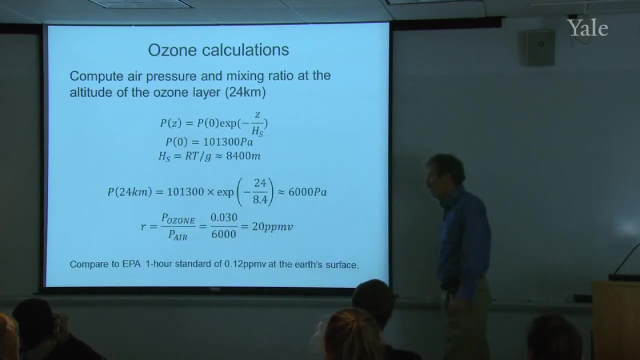 I would and I get a value of about 6,000 pascals for the air pressure up here And then I can simply put that into a ratio of the two pressures to get the mixing ratio in the common unit. So I put in that value of 30 over 0.03, over 6,000, I get. 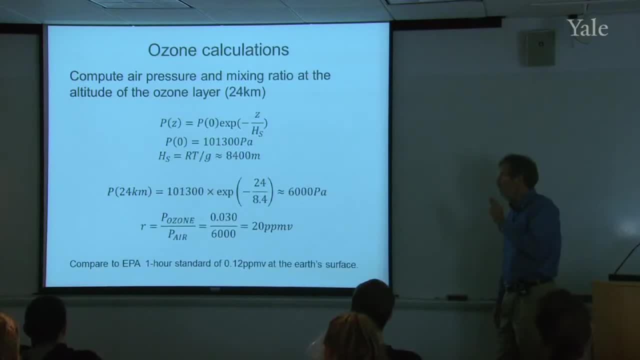 20 ppm And then I put in that value of 30 over 0.03, over 6,000, I get 20 ppm for the ozone mixing ratio in the peak of the ozone layer. Pretty straightforward calculation. Had to find out how much air was there and then form the. 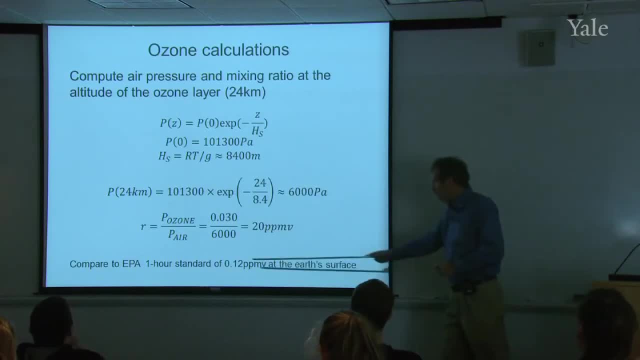 proper ratio and get it in the proper units. Now compare this with what we were talking about last time. The EPA one-hour standard for ozone in the boundary layer where we live was 0.12 in those same units. So the ozone concentration in the ozone layer is about 200. times the EPA one-hour limit, just to give you a relative sense for that. So if we were up there that would be really tough for us to breathe. that in Now remember. however, there's not enough air to keep us alive anyway at those altitudes, but the ozone concentration is. 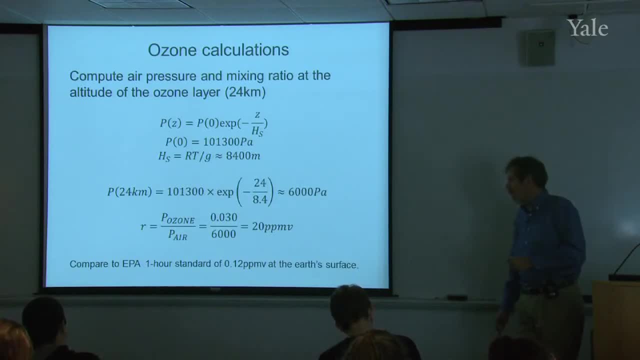 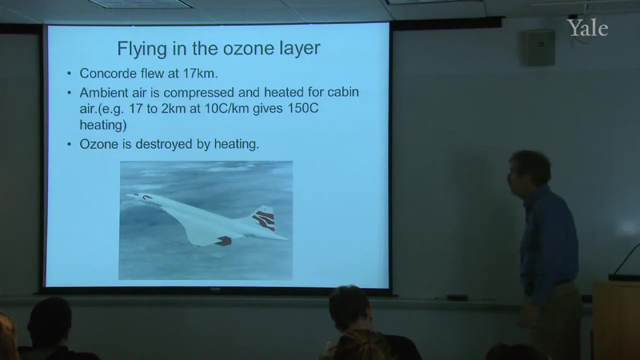 quite large as well. So that's interesting. That's an inhospitable environment up there at that altitude. Any questions on that? But it is possible, or it wasn't until recently possible, for us to fly at those altitudes. So the Concorde, this beautiful supersonic, 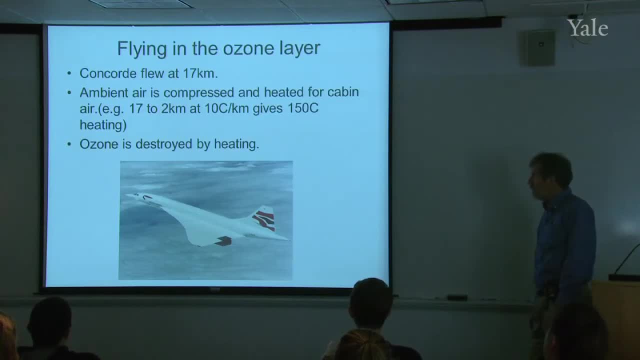 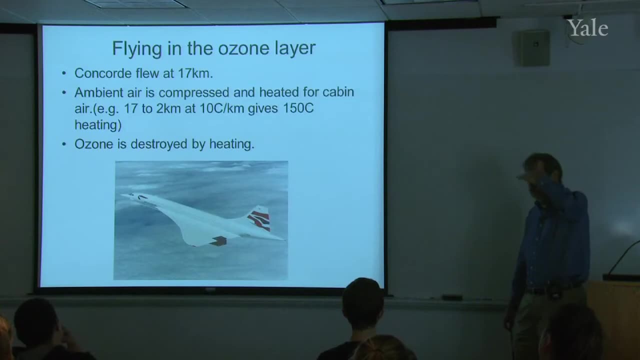 commercial airliner which stopped flying a couple years ago. It flew at an altitude typically of 17 kilometers, which isn't quite at the peak of the ozone concentration, but it's definitely up in the ozone layer. There's no doubt about that. 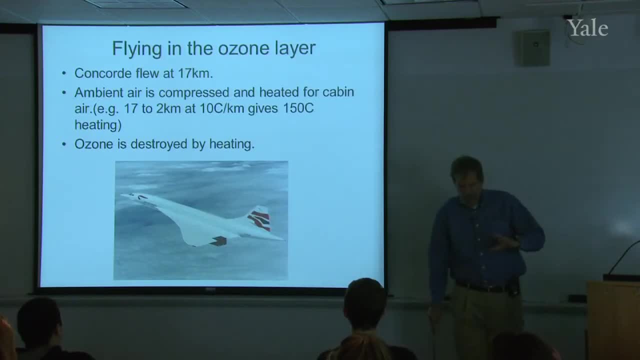 And of course you have to refresh the cabin air. You can't just lock the cabin doors and expect everybody to live off that cabin air until you get to your destination, So your aircraft can continually draw in air from outside to flush the cabin and give you fresh air. 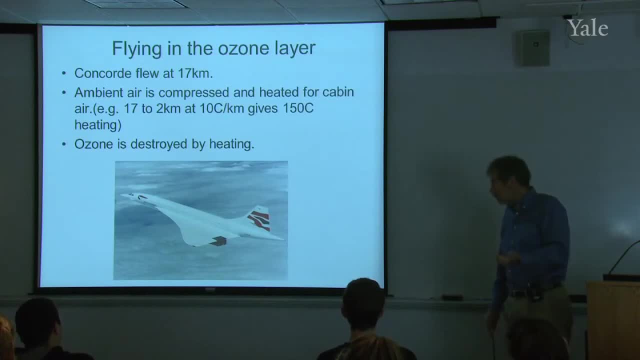 The question is: how do you do that in this case? Remember, though, that there's two problems. First of all, there's very little air outside anyway, so you're going to have to compress it with some kind of a pump before you can put it into the cabin so people can. 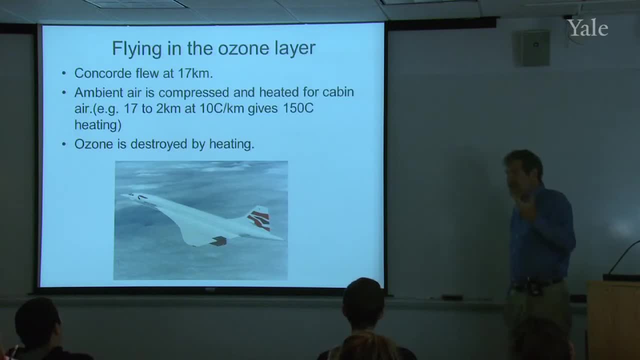 breathe it and that's going to be a big compression. Let's just think about this for a minute. So if you're flying at 17 kilometers and you want to get that air out, That air compressed to cabin pressure, Well, first of all, what cabin pressure do you normally have? 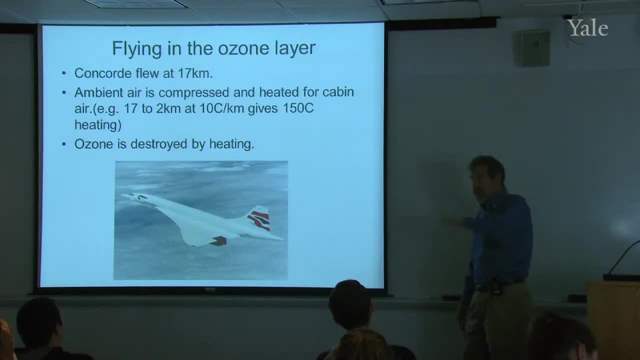 Airliners don't usually keep you at sea level pressure If you're taking off from New York City. as you take off, the pressure in the cabin will drop as you climb, but they'll usually only let it drop to maybe an equivalent altitude of. 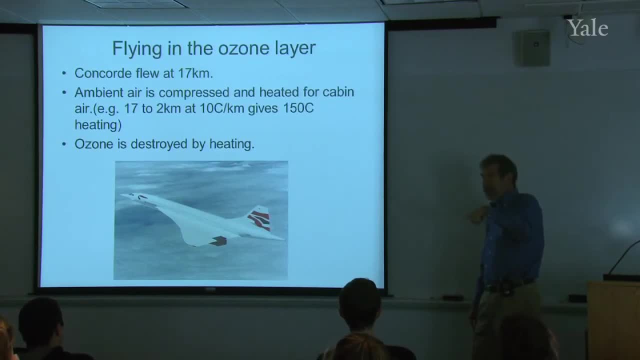 6,000 feet, something like that, and then they couldn't let it go any lower or you'd start to have trouble breathing. but they don't keep you at sea level. So I'm going to assume that for this calculation, that the aircraft. the cabin altitude- what's called the cabin altitude- is going to be kept at 2 kilometers. It's about 6,000 feet above the surface. In fact, you're flying at 17 kilometers, so you've got to. take air and compress it, just as you would if you took a parcel of air from 17 kilometers and brought it down to 2 kilometers. it would compress adiabatic compression- we've talked about this over and over again- and it would heat as you compress it. 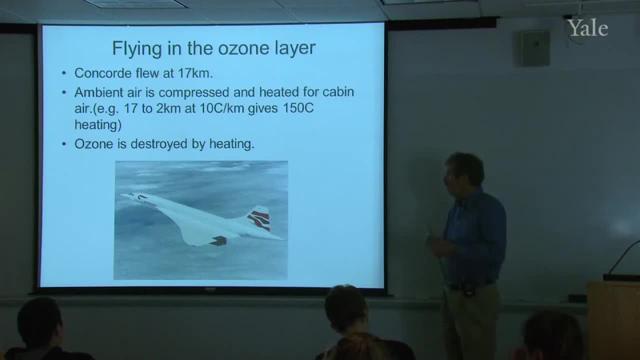 So when you put it into that pump and compress it, it's going to warm up, and how much? Well, this is a calculation you can do in your head. You know, the adiabatic lapse rate is about 10 degrees per kilometer. 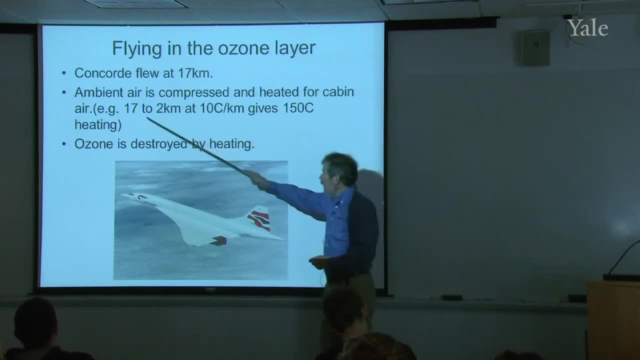 Actually it's 9.8, but I've rounded it off. That's a difference in 15 kilometers. So essentially you're going to get 150 degrees Celsius warming when you compress that air about ready to put it into the cabin. 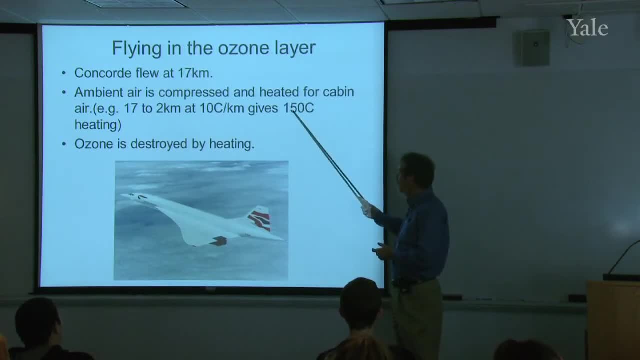 Now you're going to. it started off pretty cold, but still that's going to be really hot air. Two things I've got to say about that. First of all, the convenient thing is that that temperature will destroy the ozone. So just by compressing the air, getting it ready to put, 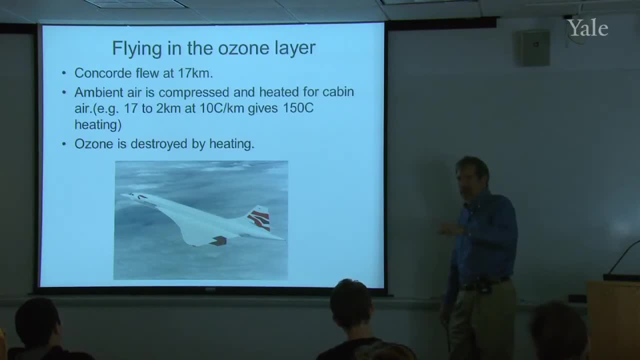 into the cabin, You're going to kill off that ozone automatically, So that's pretty convenient. But then, remember, you're going to have to cool it a bit before you put it into the cabin, So you're going to put it through another heat exchanger. 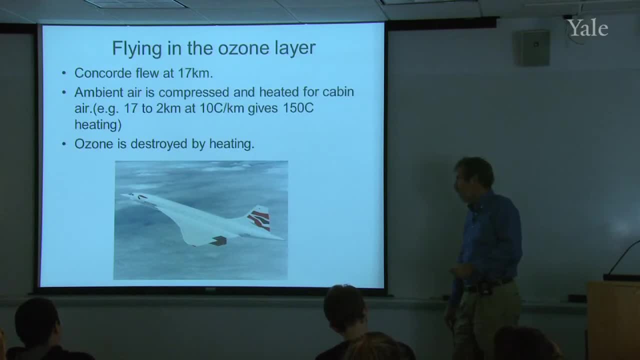 cool it back down and then you'll get the air to stick into the cabin. If you don't get it all out, you can pass the air through a activated charcoal filter and that will remove any remaining ozone that's in the air before you put it into the cabin. 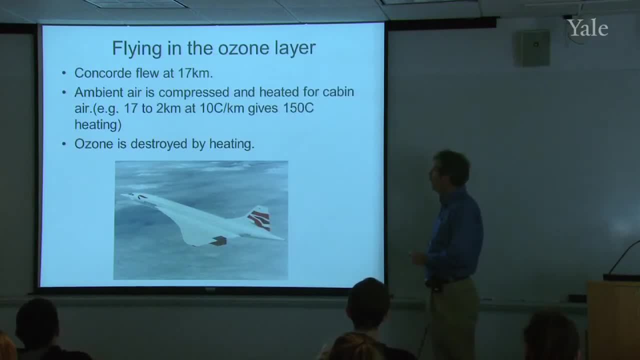 So it is possible. It's possible to fly at those altitudes right in the middle of the ozone layer, but that's how you have to do it. Any questions on that? Yeah, Why would you want to fly at that altitude? It turns out it has mostly to do with the 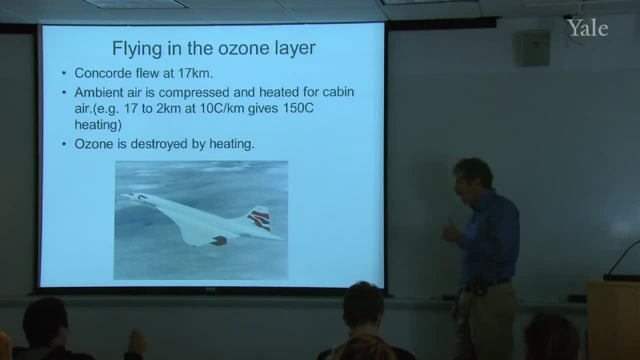 efficiency of the engines. In fact, that's true with subsonic aircraft as well. The reason they fly quite high- 35,000 feet. 37,000 feet- is because the engines are most efficient at that altitude, And for this aircraft, the more efficient altitude, the 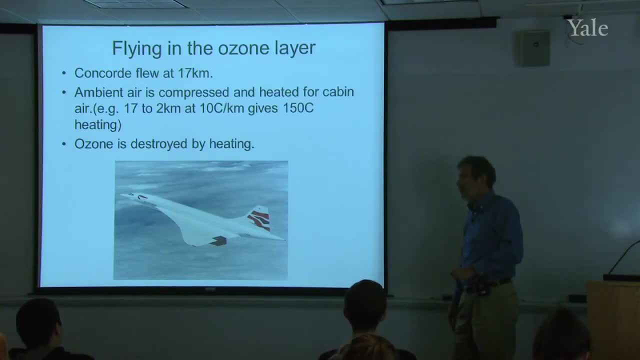 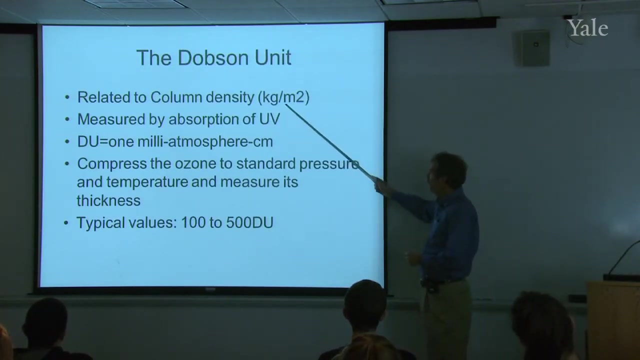 faster. it was even higher at 17 kilometers. Anything on that? OK, maybe that's a little tangential point, but this thing called the Dobson unit is a column density. We could write it. In fact, I wish that they had chosen the unit of kilograms. per square meter. You'd simply integrate top to bottom in the atmosphere and say how many kilograms of ozone are there In each square meter of footprint for that column that you've integrated over. But for historic reasons they didn't do it that way. 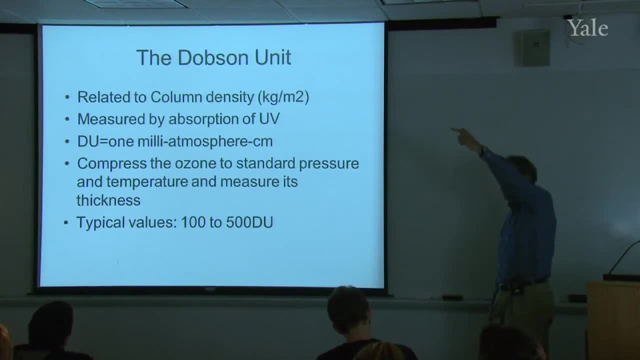 This is typically measured by looking at light coming from the sun and see how much ultraviolet light reaches the surface of the Earth, And that'll tell you how much ozone there is in the column. What they're using for the Dobson unit is this definition. 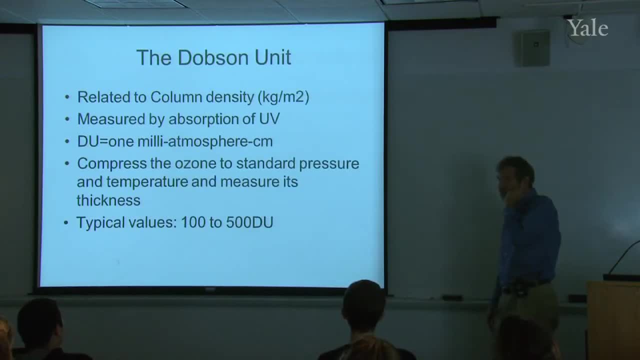 It's one milli-atmosphere centimeter. OK, That's the scientific definition of a Dobson unit. And here's how you think about that. You take all the ozone in the column, You compress it to standard temperature and pressure. 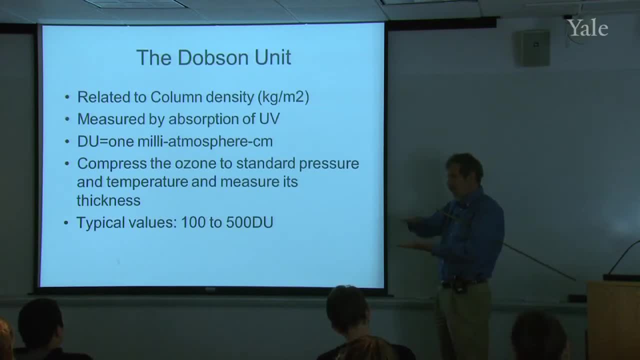 That is one atmosphere of pressure and 0 degrees Celsius. and then you measure how thick that layer would be composed just of ozone, and you measure that in thousandths of a centimeter and that is your Dobson unit. That's the Dobson unit value. 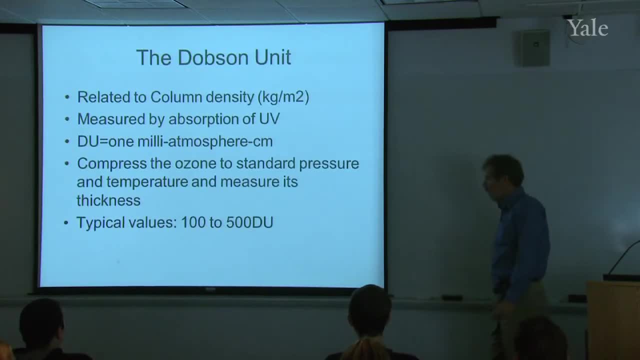 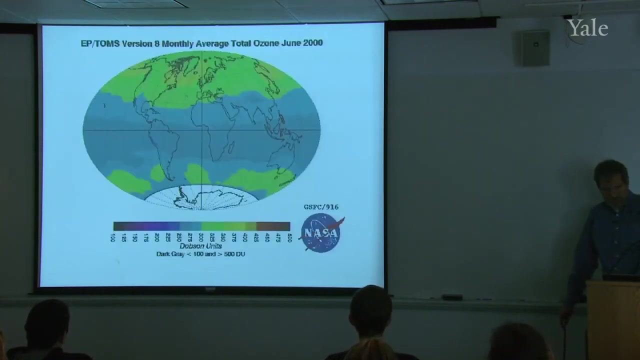 And I'll be showing you this kind of data. Typical values for the Earth atmosphere run from 100 to 500 Dobson units, depending where you are around the world, But that is normally. the Dobson unit is what we use to describe to each other how much ozone. 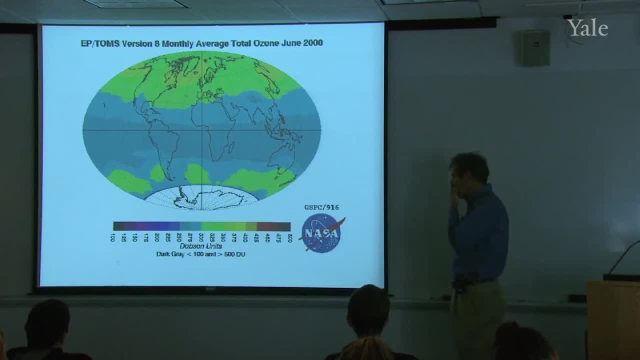 there is in the atmosphere. So, for example, you'll see a diagram like this from NASA. It's a map of the world, Some areas blocked out because they don't have data. We don't have data from here for this particular time of. 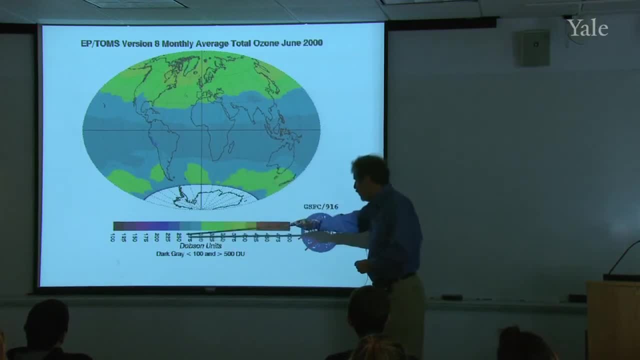 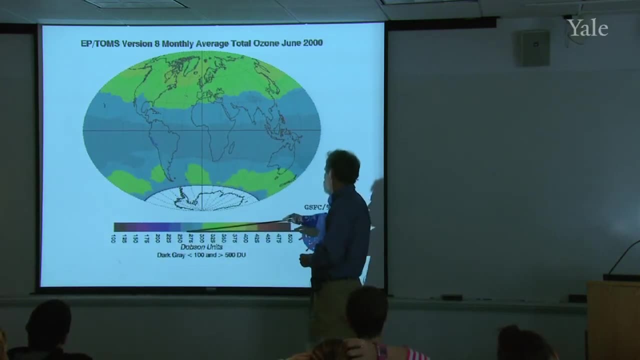 year, but the scale is in Dobson units. So in the tropical regions you're getting values about 250, 260 Dobson units. In the green you're getting values maybe 325, maybe in some areas even 350 or 360. 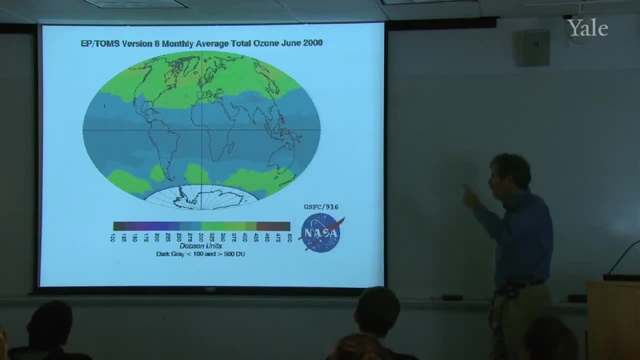 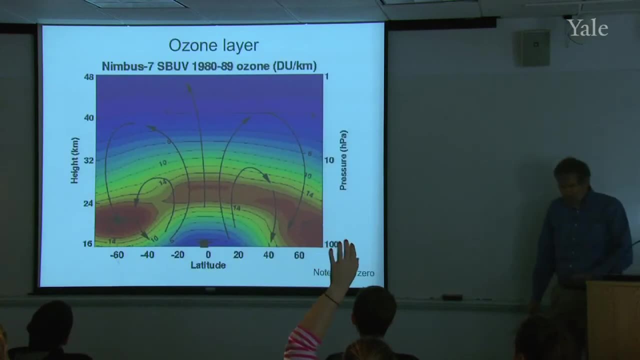 So that's the way we represent column integrated ozone. on this subject, We can also get vertical profile information, either by direct in situ measurements or by looking at light passing across the Earth, the Earth's atmosphere, horizontally. This gives you some idea of where the ozone layer is as a function of latitude. So here's latitude: North pole, south pole, equator altitude. But notice the offset zero. This isn't the ground. This is starting at 16 kilometers right. So the ozone layer at higher latitudes is at an altitude of. 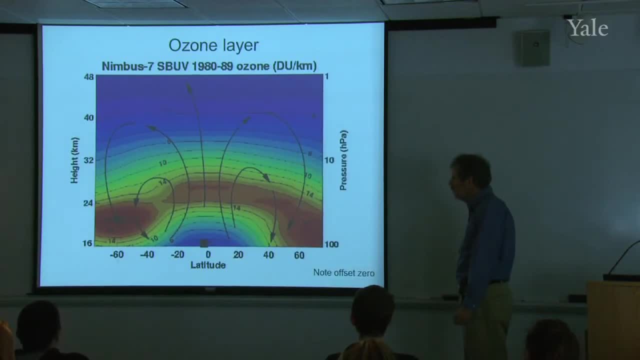 about. it peaks at an altitude of about well, 20 kilometers, 18,, 19, 20 kilometers, But near the equator it's up around 25, 26 kilometers. I think we expected this because remember the tropopause. 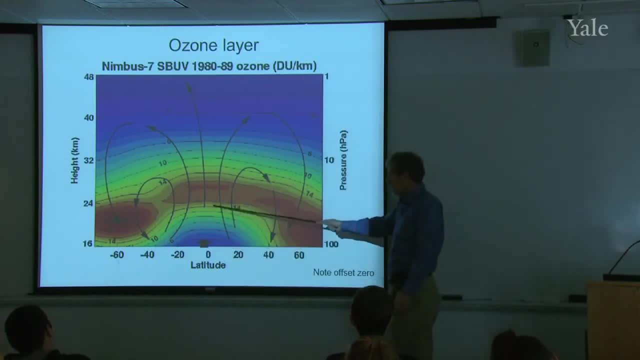 has the same kind of a structure. It's higher in the equatorial regions and lower in the equatorial regions, And it's higher in the equatorial regions and lower in the polar regions, And so the ozone layer is about the same place in the stratosphere. but the stratosphere starts at a different level, So it's lifted in a sense relative to the surface of the Earth in the equatorial latitudes. Part of the reason why there is that difference is because of a broad circulation that takes place in the stratosphere. 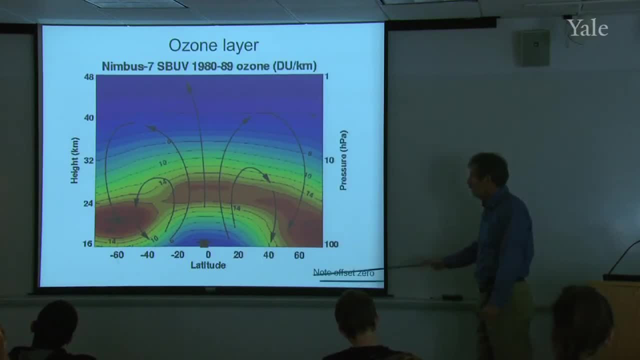 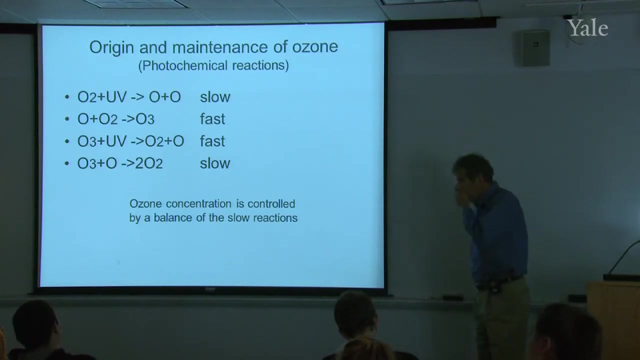 called the Brewer curve Dobson circulation, which I won't talk about. But this artist has reminded us that there is this broad, slow circulation in the stratosphere. So why do we have ozone in the stratosphere? This is the basic chemistry of that. We know we have a lot of O2 in our atmosphere. it's the second most common molecule and occasionally a high energy photon will". No problem here will come from the sun. A high energy ultraviolet photon will dissociate that diatomic oxygen into two oxygen atoms. Doesn't happen very often because it needs a high energy photon to do that. But then you've got some free oxygen atoms floating around And when you have that that'll quickly combine with an O2 molecule to form ozone. That's a fast reaction. 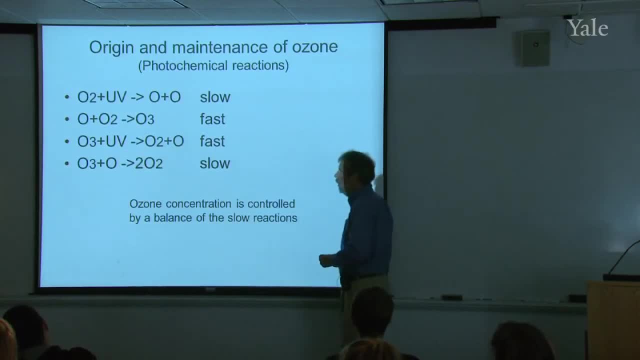 But equally fast is that other ultraviolet photons. they don't have to be as energetic as this one. These can be in the near UVA, for example. the near ultraviolet will dissociate that back to this again And that's fast. 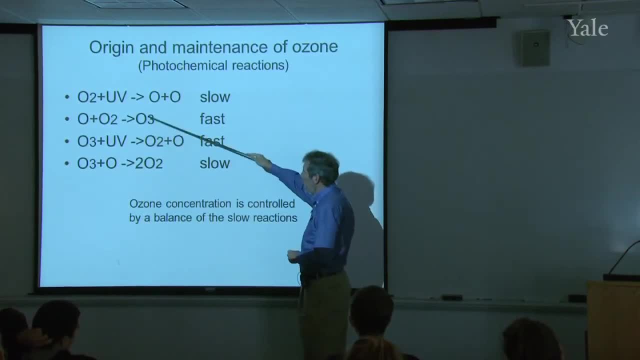 So what you've got is a rapid recycling going on between that and that. that's just going on all the time in the stratosphere, But maintaining a balance here. Now, occasionally, an ozone will interact with one of these atoms and go back to O2, which is the common form. 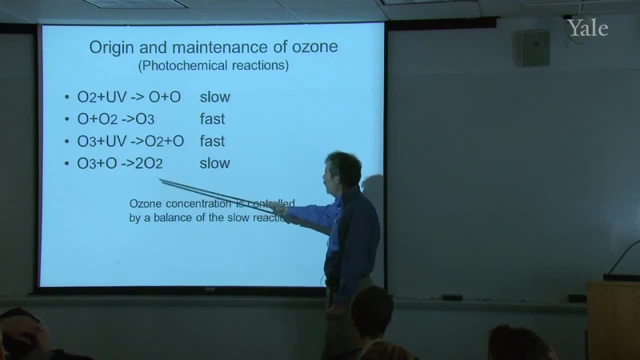 And then you've lost it. So you've lost the ozone permanently, or at least quasi-permanently. So the ozone concentration is controlled by ignoring this rapid cycling, which doesn't have any long-term effect. It's controlled by the balance of these two slow processes. 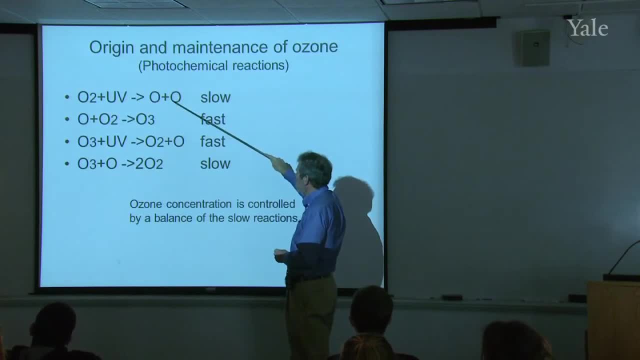 How often are you producing oxygen atoms and how often are you removing ozone and oxidized atoms back to O2?? And that would be occurring naturally because we have oxygen in the atmosphere and we have ultraviolet light coming from the sun. So that's the background to why there is 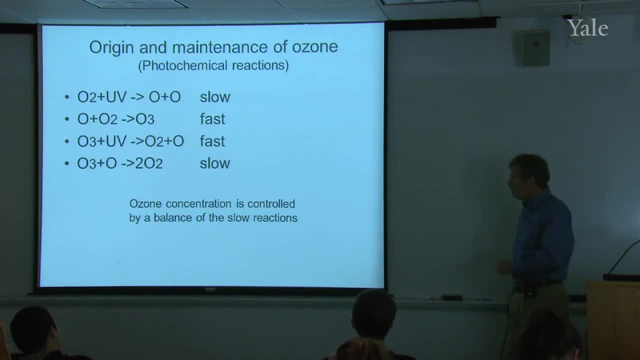 ozone in the stratosphere. The reason why it doesn't happen further down is because most of these ultraviolet photons are absorbed up there and don't penetrate deeper into the atmosphere. So it's a layer up there, because that's where these 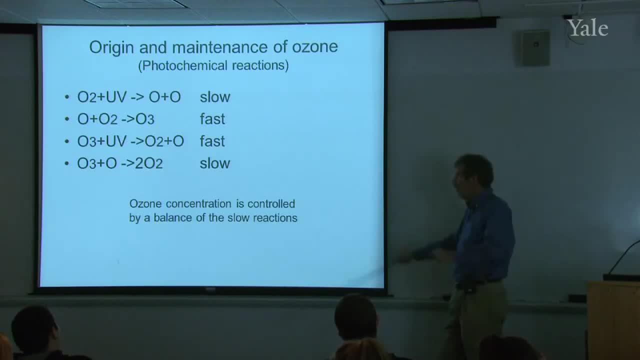 ultraviolet photons are being absorbed and doing this work, causing these photochemical reactions to take place. Questions on that. Yeah, I'm curious if there is some sort of feedback mechanism or if the two slow reactions are interconnected in some way, because I guess, if you have more free oxygen, 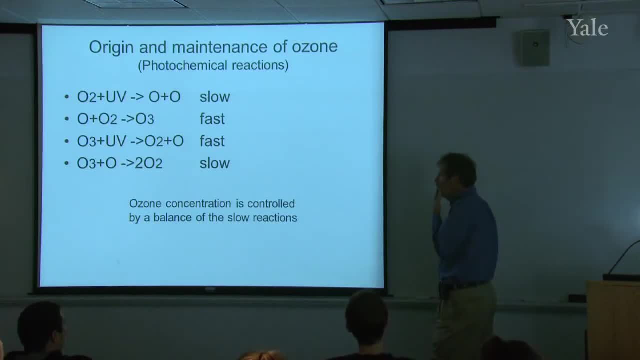 atoms that would allow the second process to occur more frequently. Well, you'd have to write down the rate equations for these to answer that question, which I'm not prepared to do, But this obviously will. you know, a chemical reaction depends on the rate at which it goes forward, depends on how 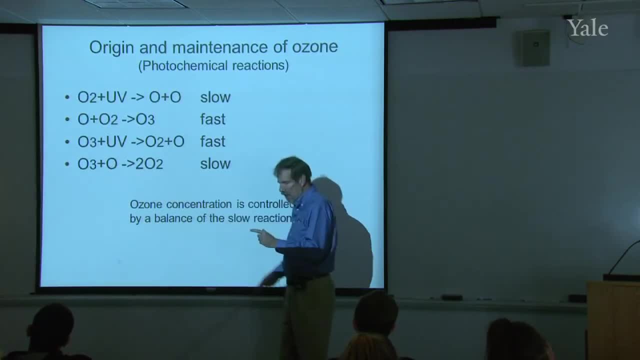 much of this do you have? and how much of this do you have, and how often are they colliding To allow the reaction to go forward? So I think your instinct is right that these are going to depend on the concentrations that you have. 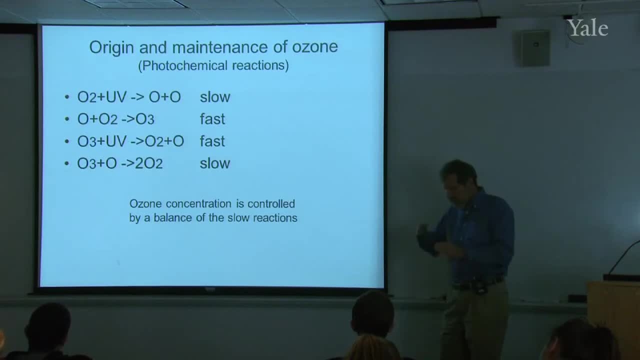 So, just like our tank experiment, the loss rate was proportional to how much you have. And that's what. in a system like this, where the generation term is independent of how much of this you have, but the loss rate is proportional, you're going to come to an 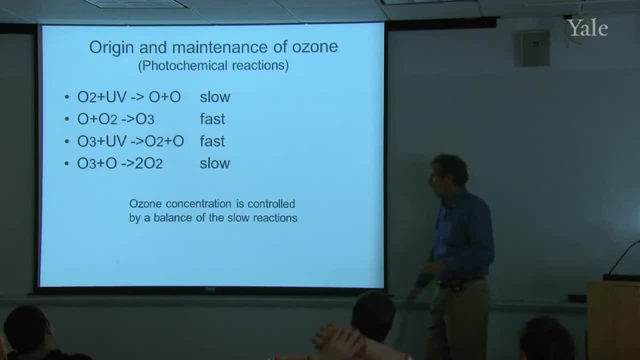 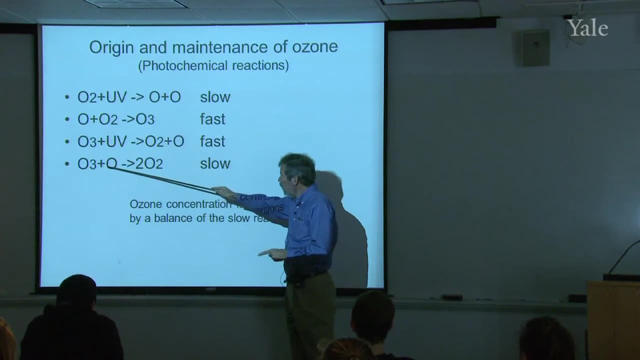 equilibrium, just like we did in the water tank, and that's what I'm implying here, that you've got the kind of balance between a source which is just there and then a sink which is dependent on how much you have. 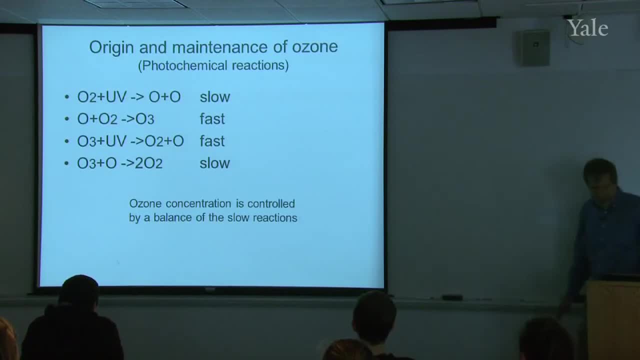 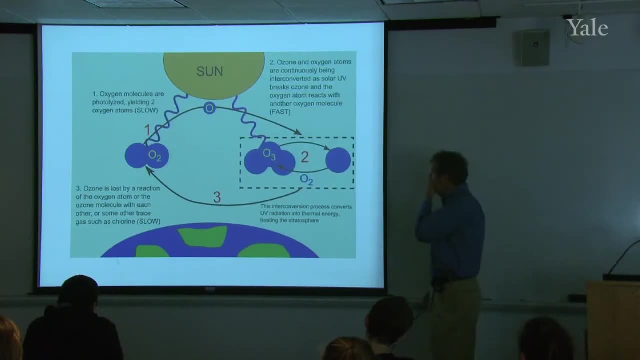 And that will give a natural equilibrium. eventually- And this is a cartoon showing that, So the sun is playing a role- Occasionally it will dissociate O2 to form a symbol O, an O molecule, And then you get this rapid recycling between oxygen atoms. 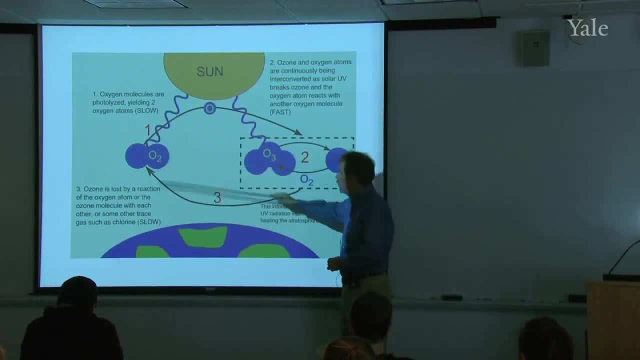 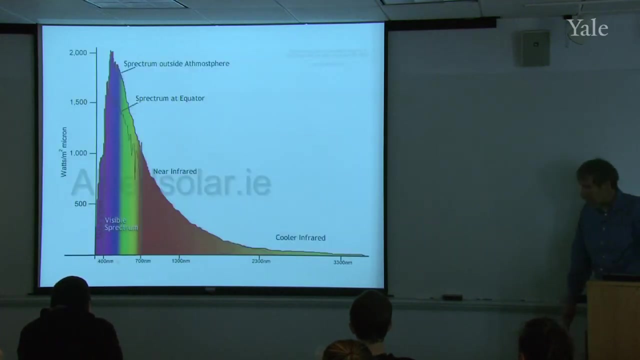 and ozone, and then occasionally you'll go back just to the O2 again, And the control of how much you have is primarily these processes, not this. This is just a rapid recycling of the two types of oxygen. Now to remind you about the spectrum of radiation coming. 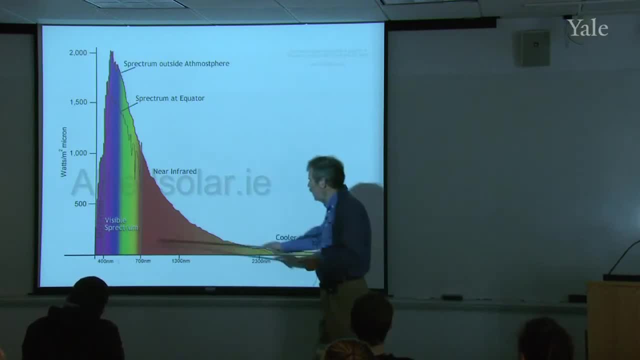 from the sun. I show you this, You've seen it before: The visible spectrum is here the infrared. We're really interested in the ultraviolet over here in today's conversation, which starts at 400 nanometers wavelength and goes shorter than that. 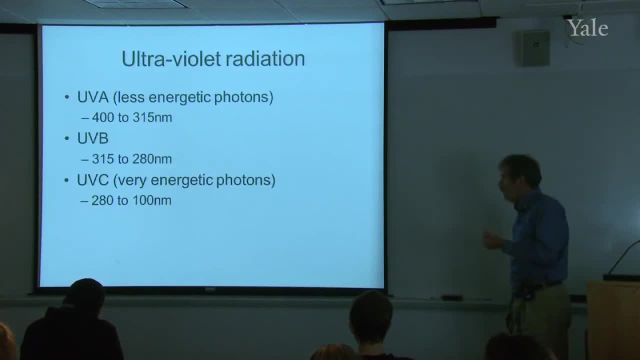 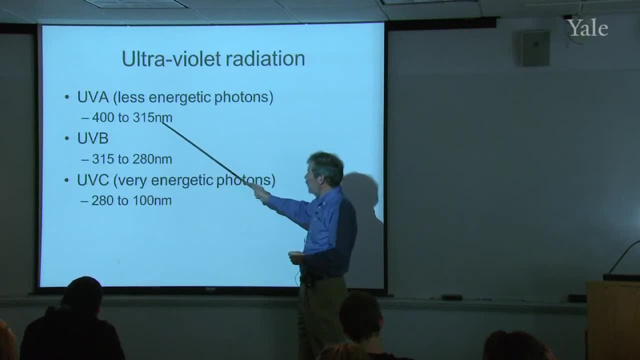 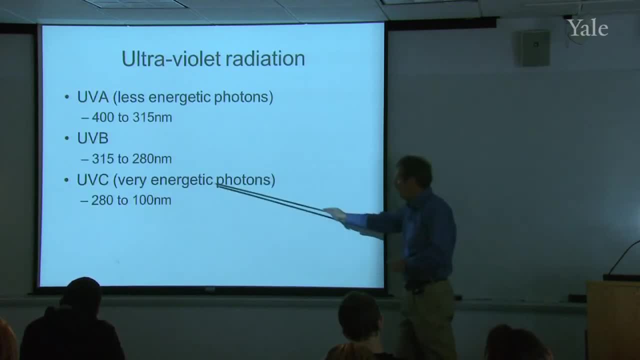 Defined by the UVA, Defined by the UVA And UI is the enrichingray ordered state temperature. Now, when study like this here in дN, I think if you did it you get the kind of level ofρά that you expect over a hundred years or so. 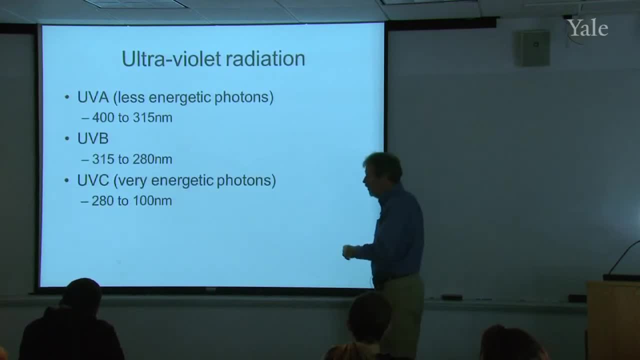 And there's a lot damaging. In fact, it's used in doctor's offices to clean surgical tools. You put it into this autoclave, which will put UVC on your instruments and it'll kill anything that's there very, very quickly. 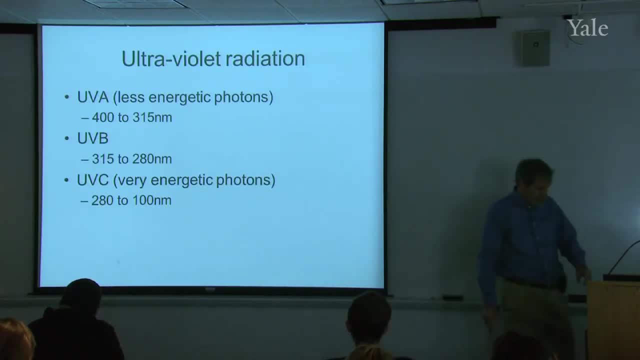 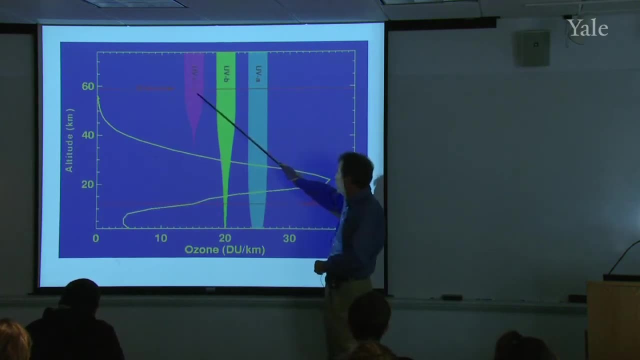 It's very damaging, very damaging radiation. And so here's the fate of UVA, UVB and UVC. Some UVA comes through. Half or more of the UVB is absorbed in the ozone layer. Plotted on top of this, this is altitude and Dobson units. 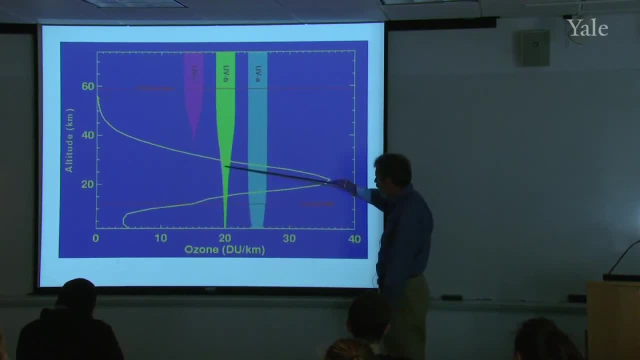 per kilometer to get where the ozone layer is. So about half or two thirds of the UVB is absorbed by the ozone And almost all- thankfully almost all- of the UVC coming from the sun is absorbed by the ozone layer, So it's a very good protective shield for us. 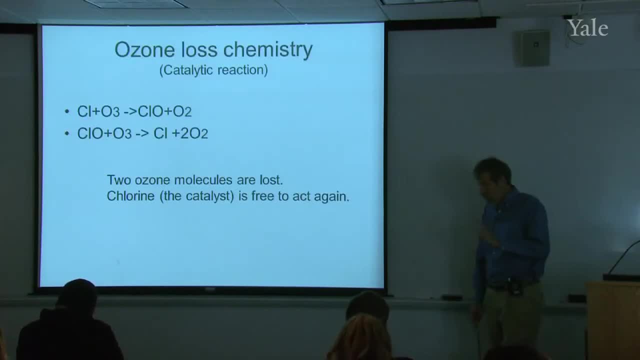 Now, what could be changing this natural ozone layer situation? Well, this is the current theory for it. It involves a catalytic reaction, primarily using chlorine atoms. Now, bromine will do this as well, and there's some bromine in the atmosphere, but I'm going to focus strictly on 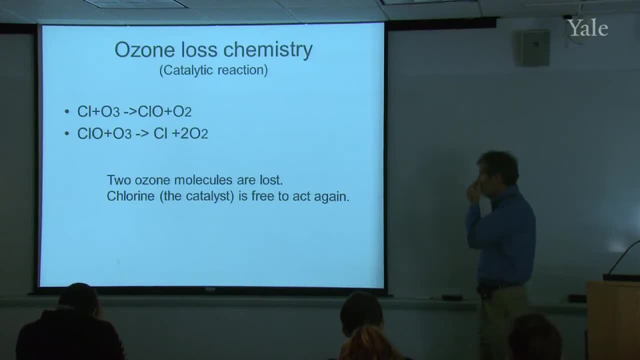 the chlorine And notice how this reaction works. So you have a chlorine atom reacting with an ozone molecule. it goes to ClO, it oxidizes the chlorine and gives you back O2.. And then, quite soon after that, you'll take this ClO and 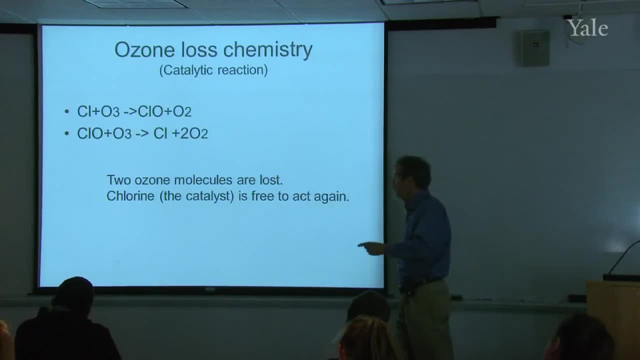 react it with another ozone molecule. That'll give you back the Cl that you started with and you have two O2s, two regular diatomic oxygens. So look, the ozone is gone. In fact, two ozones are gone and you've got your Cl back. 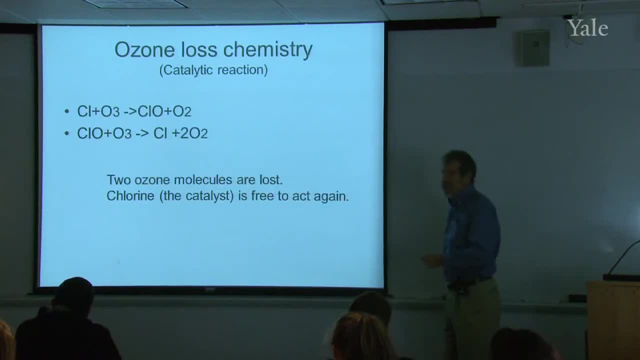 ready to do it again. So this is a catalytic reaction where the catalyst here is the chlorine atom. It can be used over and over again to destroy ozone molecules. In this way, Two ozone molecules are lost and the catalyst is free. 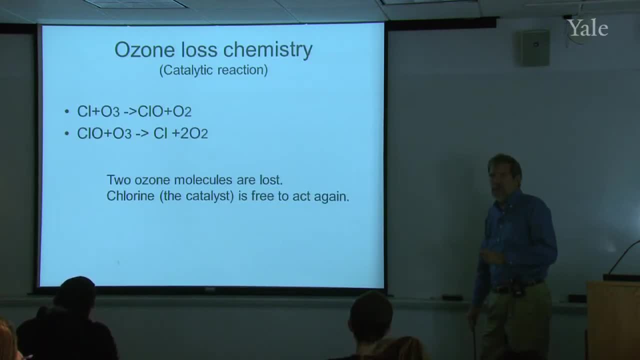 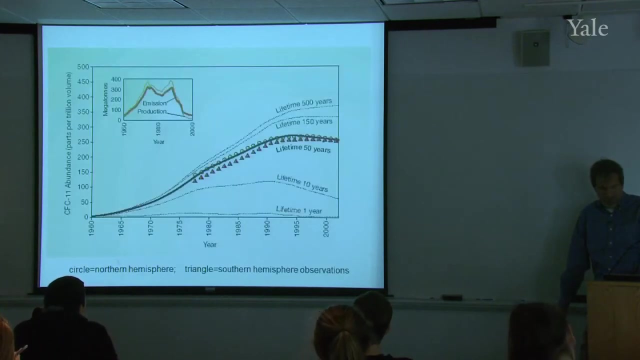 ready to go back and do it again. That's the idea of what's today, now that we have a measurable chlorine concentration in the atmosphere. this is why we think the ozone layer is decreasing. Questions on that. So up here in the inset is the emission. 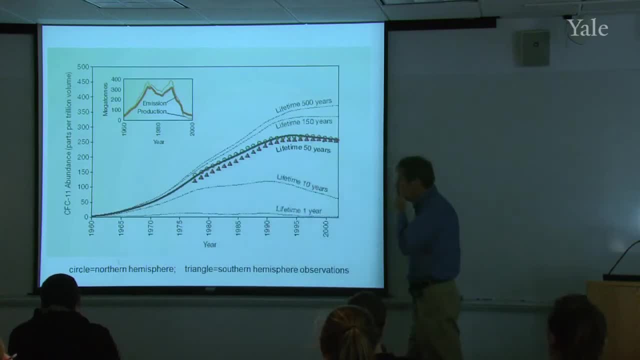 This is an example: See CFC-11,, one of the chlorofluorocarbons, and here's the emission rate for it in megatons per year, starting in 1960, going up to the year 2000.. 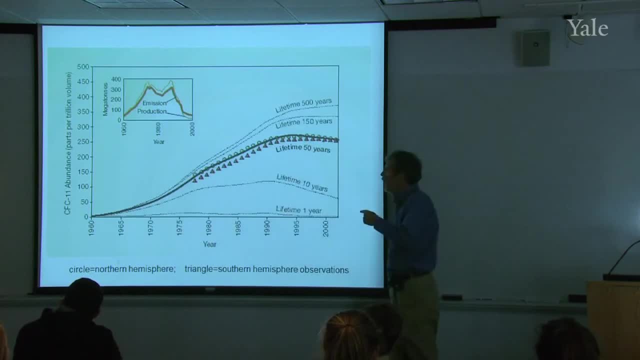 So you see there was a rapid rise in it as it was being used in refrigeration And when you put it into a refrigerator it may be contained for a few years, but eventually it leaks out or it's torn. Someone tosses away the refrigerator and it gets a. 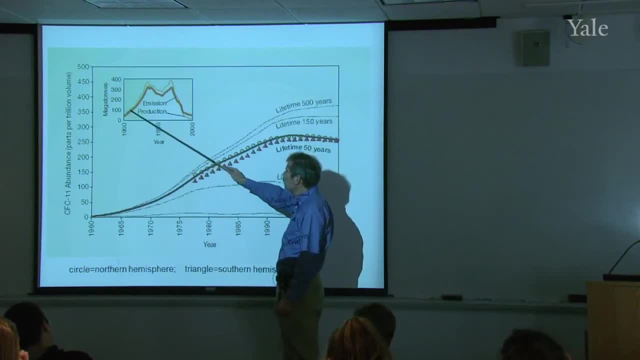 leak and it goes to the atmosphere. So almost everything you produce eventually makes its way into the atmosphere. The Montreal Protocol that I'll talk about was here, where you begin to see, finally it decreased, But because it's a long-lived molecule. here's the CFC. 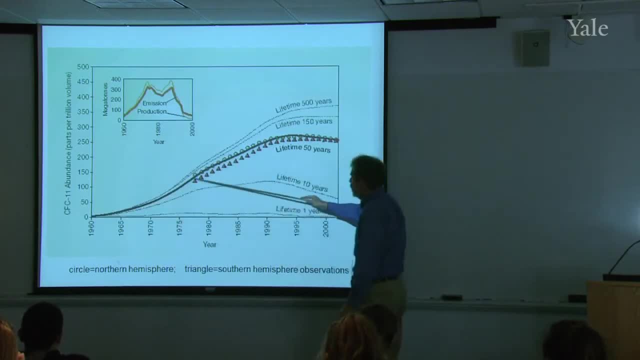 abundance in the atmosphere. It increased through this period of time. We've stopped putting it in, but it's still there. It has a lifetime. From this data, it looks like the lifetime is about 50 years, And so it's going to take probably another 50 or 100. years before we see much of a decline. Thank goodness we've stopped putting it in. But it's not going to decrease to zero just because we've stopped putting it in. It's going to be stored in the atmosphere for a while. It has a long lifetime. 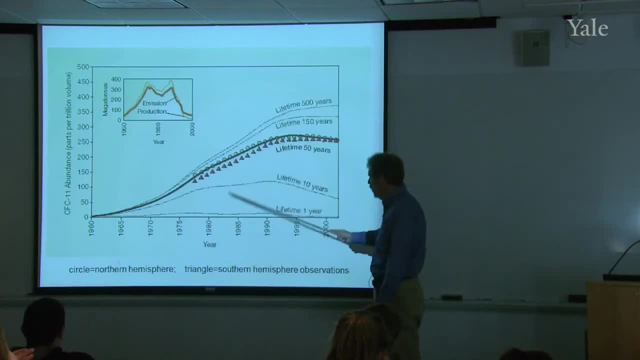 The circles are data from the Northern Hemisphere and the triangles are data from the Southern Hemisphere, But they're pretty much the same, So the two hemispheres. this stuff gets mixed back and forth. Probably most of it was put into the atmosphere in the Northern Hemisphere, but now it's mixed to be pretty much equal in the two hemispheres. Questions on that. Here is the global averaged total ozone change in percent Starting back in 1965.. Around 1980 is when we began to see the rapid decrease. But it's not huge. Notice that it's leveled out today and it's only about 4% below where it started. So this global decrease in ozone is, I suppose it's something we should be concerned about, but it's not a huge factor. 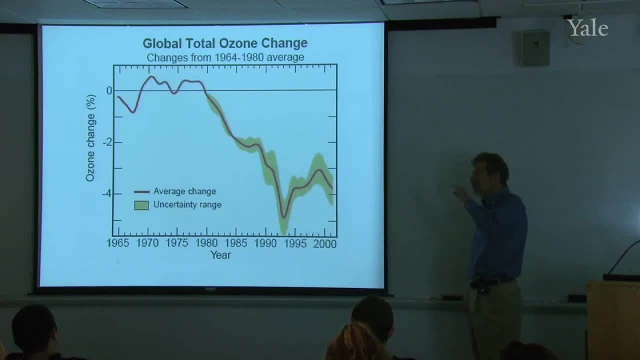 And it doesn't look like it's going to get any worse now that we've stopped putting CFC there. Right, Right, It's going to freeze into the atmosphere. So it's a concern, but not, I would say, a terribly. 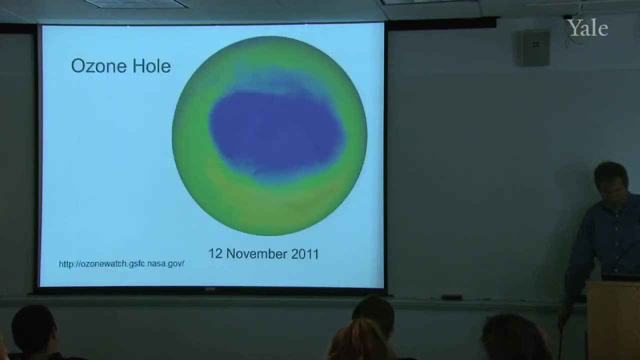 difficult one. But then there's this ozone hole that I'll spend the rest of the time talking about, And here is what it looked like a couple of days ago. You can go to this website, which I'm just about to do. I should have set this up before. 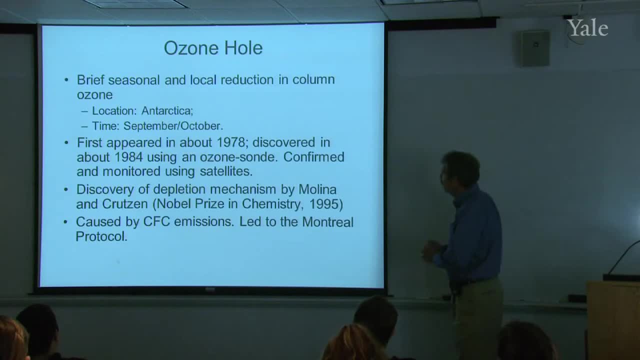 But here's a definition of it. So it's a brief, seasonal and local reduction in ozone. Location is Antarctica. The time of year that it happens each year is September or October. It first appeared in about 1978.. Apparently it wasn't happening before then. 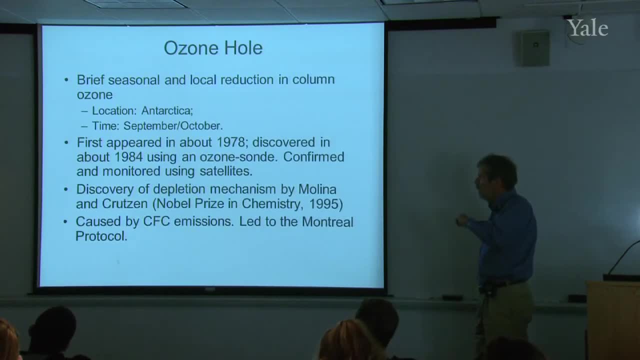 It was discovered in 1984, and then, going back and looking at old data, they found that it actually had started some six years earlier than that. The discovery of the depletion mechanism by Molina and Crutzen Was a rather remarkable scientific discovery. 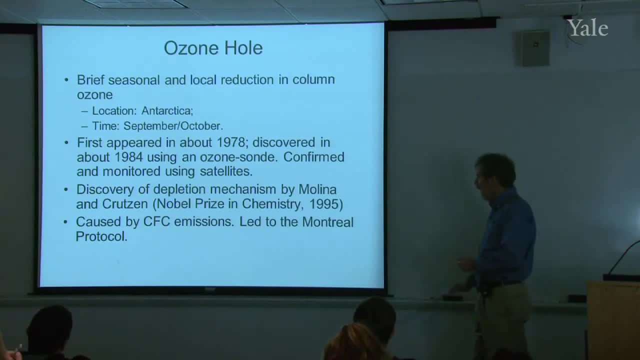 I'll give you hints of how that went in just a minute. And they won the Nobel Prize in Chemistry for that, awarded in 1995, from that discovery of how the ozone depletion mechanism works. Ultimately it's caused by these CFC emissions, which then 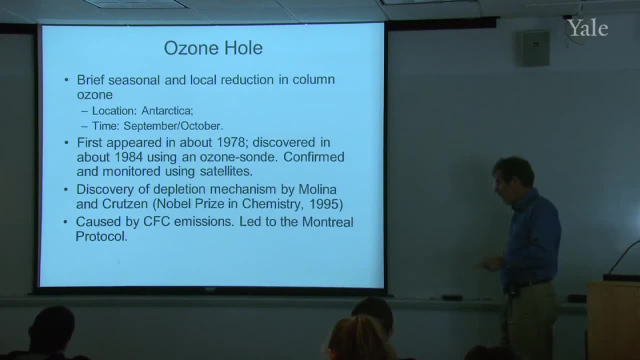 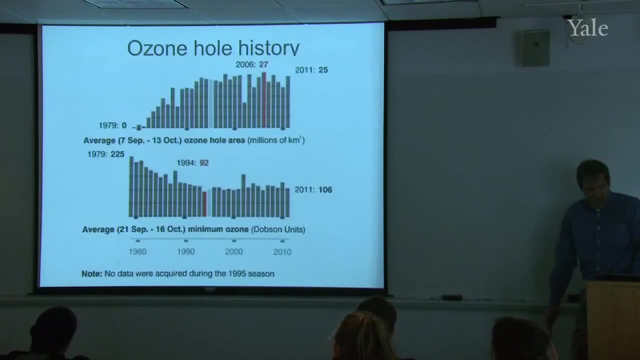 led to the Montreal Protocol, which I'll talk briefly about, A rather successful international treaty to limit the emissions of CFCs. Here's a brief summary, A brief history of it. So at the top is the ozone hole area in millions of square kilometers. 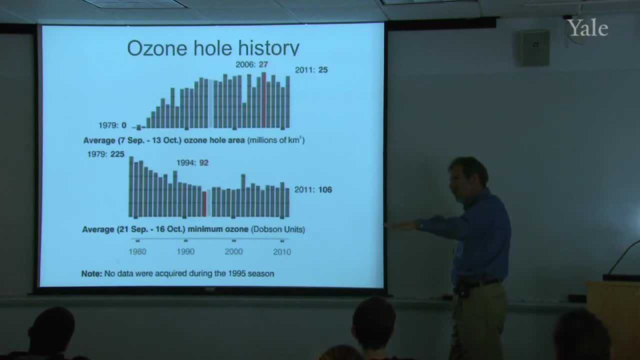 What you do is set a threshold for ozone concentration. If it's lower than that, you say you're in the hole. If it's larger than that, you're out of the hole, And then you keep track of that area. And the ozone hole was nonexistent before 1979, but 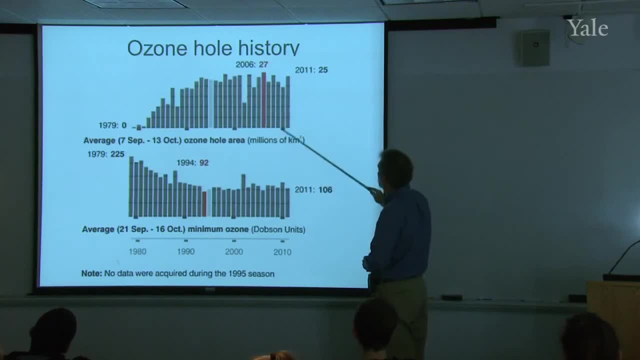 now has reached about 25,000.. 25 million square kilometers. You saw a picture of it And it's kind of leveled out. It's not getting any better, not getting any worse. And the minimum ozone in the middle of that hole is shown. 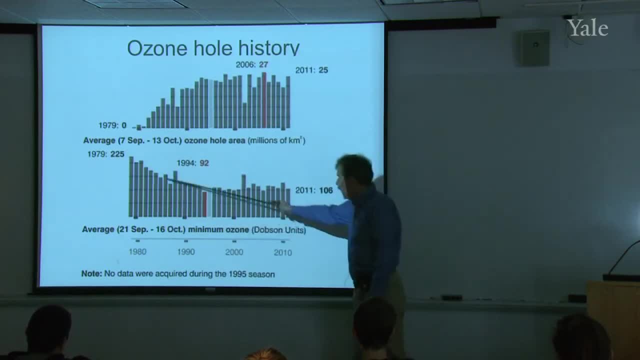 here in Dobson units, of course Getting worse, but now leveling out to a value of about 100 Dobson units- in the middle of the hole each year when it forms. So give me just a moment here to bring up the next slide. 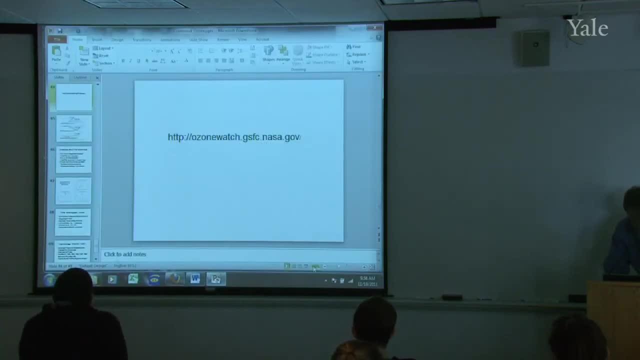 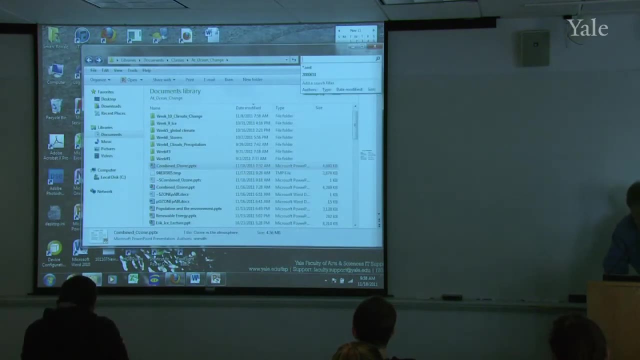 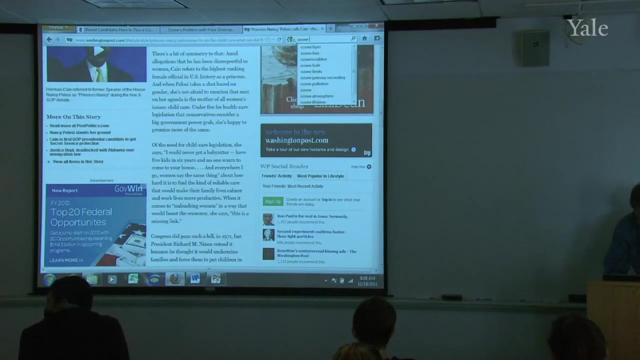 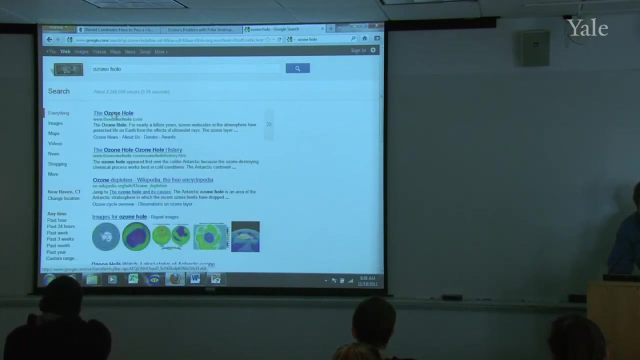 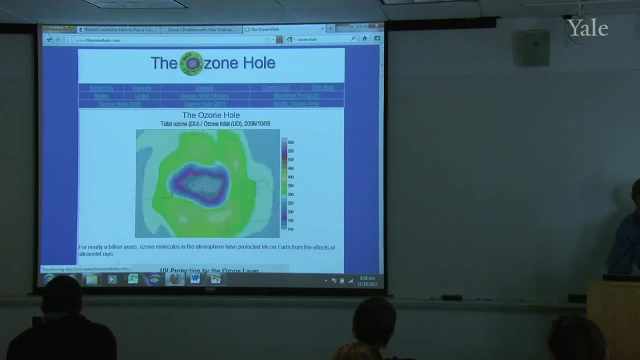 This website. I forgot to do this before. I'll just Google and find it. Yeah, that's probably it. That's not the one I want. Yeah, that's a good one, But it's not the one I'm looking for. 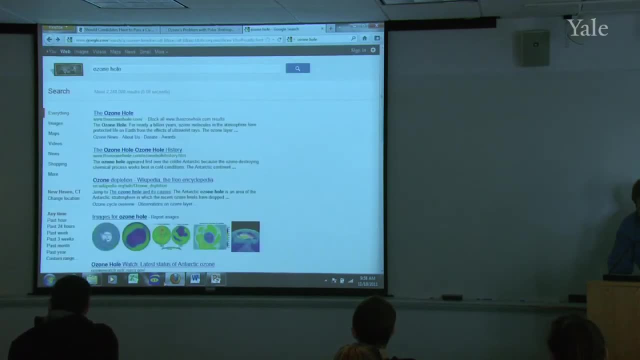 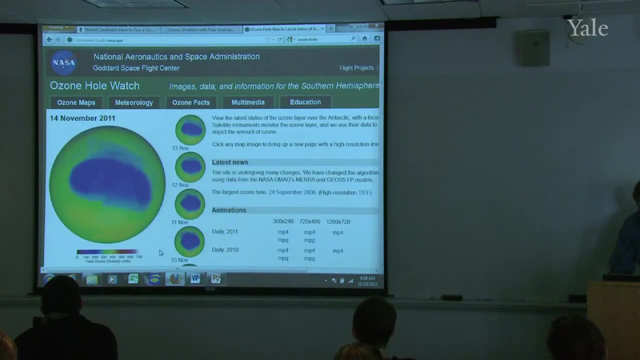 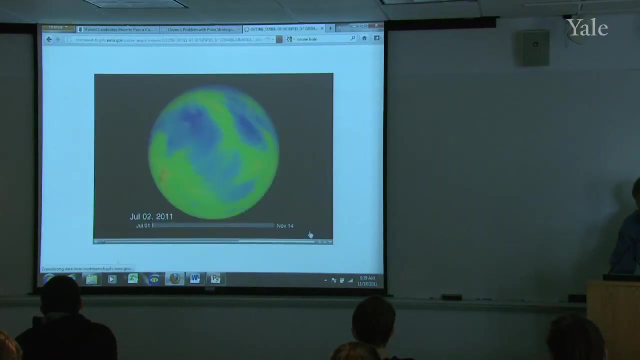 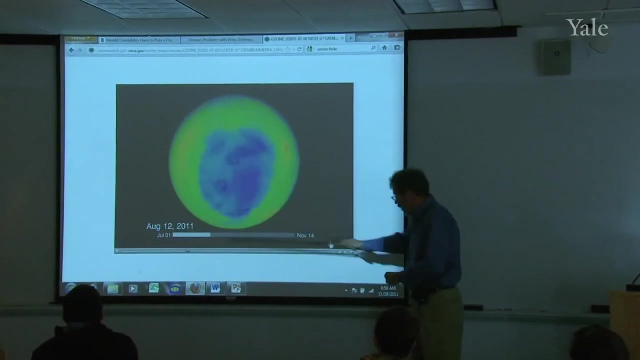 Try to find this other one. Yeah, Let's do an animation for this season. Yeah, so this is this year's oven. What is it? It hasn't formed yet. We're back in July. This is Antarctica sitting there waiting. 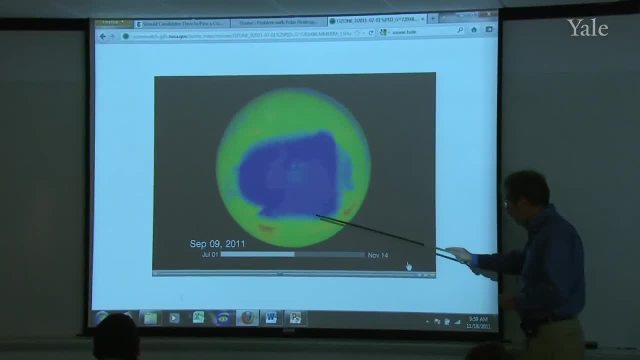 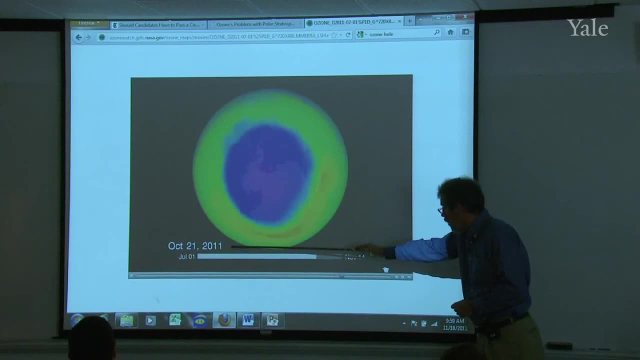 Now, when do we get into September? It's already beginning to form in the late summer, but now we're getting the ozone hole forming. October peaks in October and then it'll start to fill in. up to the present date It's starting to weaken now that we're into November. So that's the deal. It happens every year in that region. You get this large area that forms with about half the ozone it would otherwise have. Ozone depletion is about 50% in that region compared to- remember- only 4% globally. 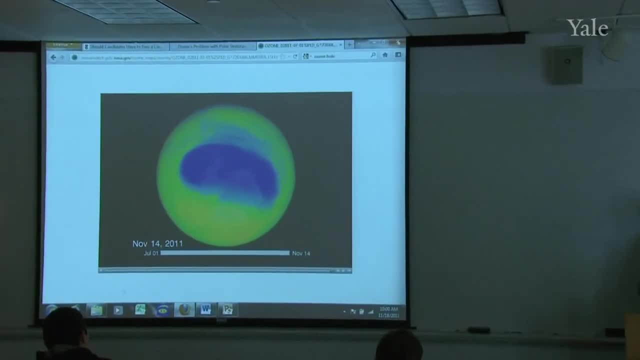 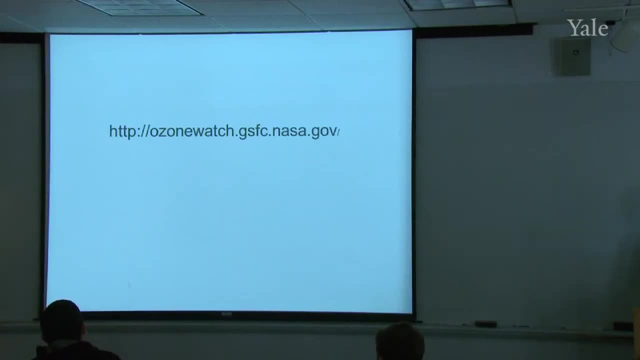 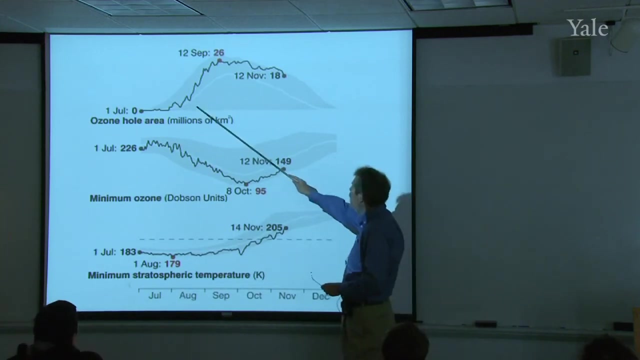 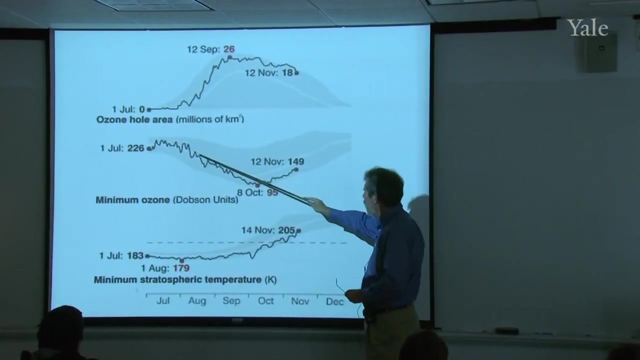 So this is a localized anomaly. You can go to that website yourself and do some other animations. So in this year then this track exit. the ozone hole area climbed up to the 12th of September. Now it's decreased. The minimum ozone dropped to a minimum. 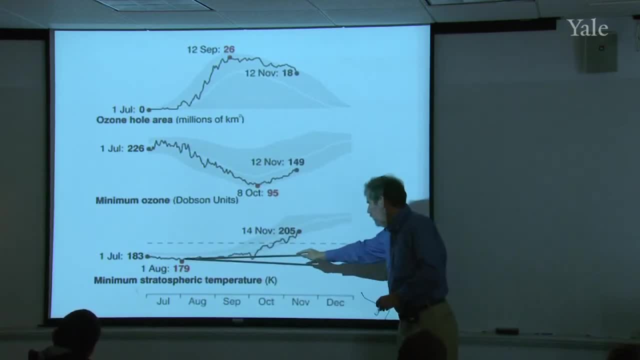 Now it's increasing Now that we're into November, And I'm going to be talking about this stratospheric temperature. Stratospheric temperature in that part of the world now, at that altitude, is beginning to climb because we're getting out. 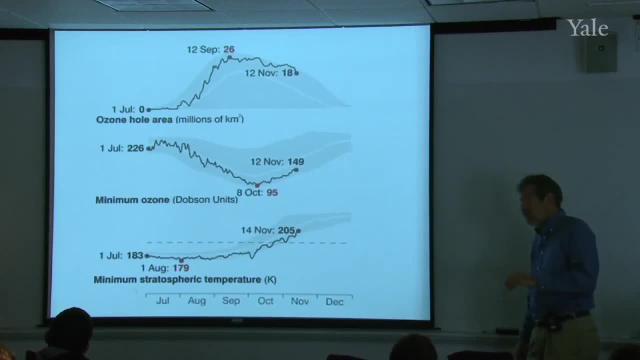 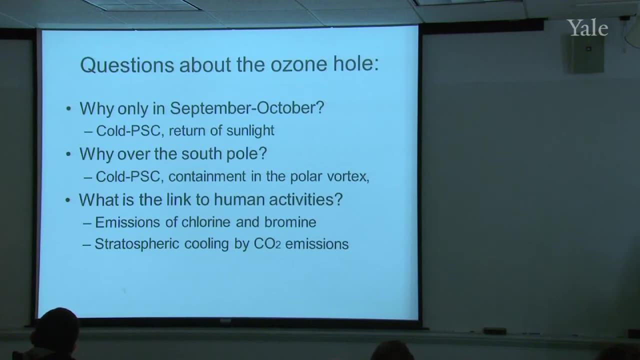 of their winter and towards their southern hemisphere summer, and I'll come back to talk about the role of the temperature in a just a moment. So I think the most curious thing about the ozone hole is why only in September or in October? Why just over the South Pole? 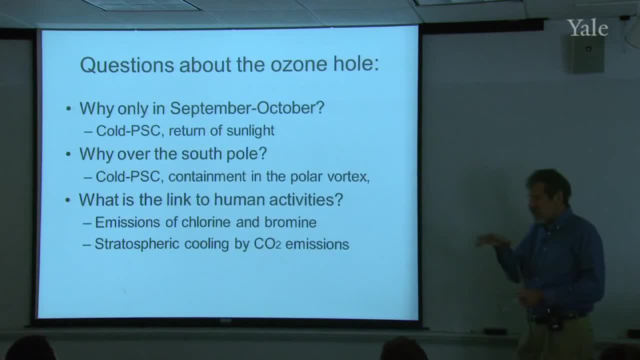 And I guess what is the link to human activity? So there's a lot of natural processes and factors controlling this, And then there's the added impact of humans and somehow they've all come together, They've all grown to these الم. And then there's the added impact of humans and somehow they've all مع. 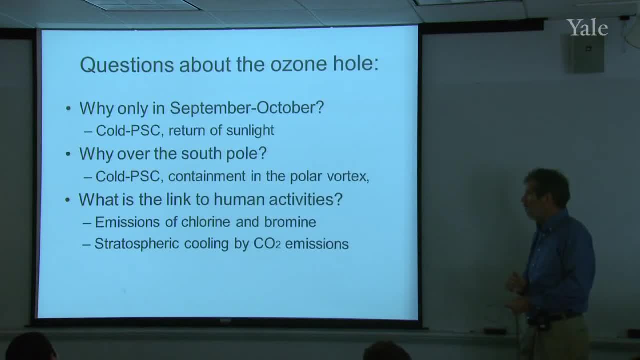 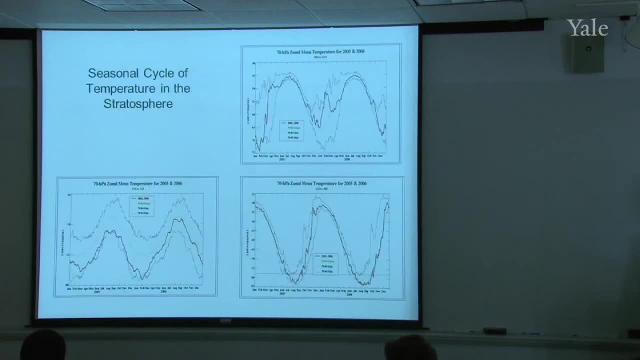 come together with обязangverts to form this curious phenomena of the ozone hole. In the few minutes I have left, I want to just try to explain some of that Now. I hope you can see this. I'll read it through for you. 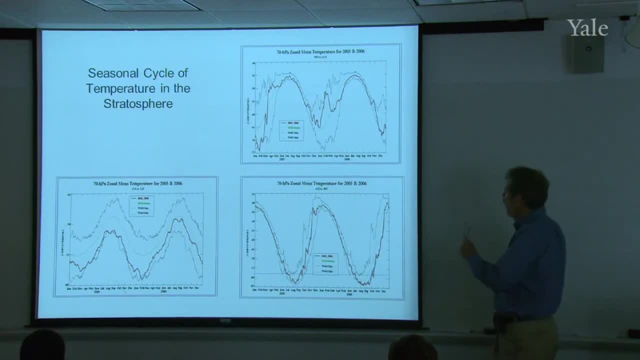 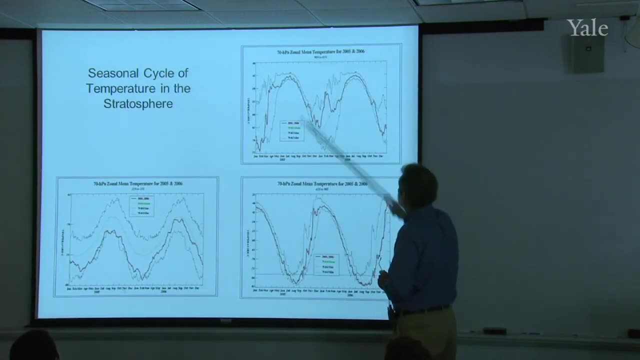 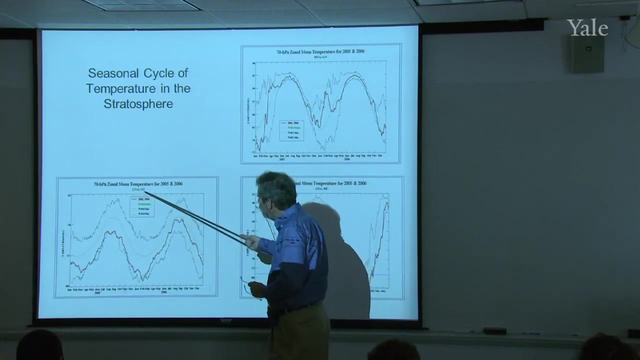 This is the seasonal cycle of temperature in the stratosphere And this is for 90 north to 65 north, So this is the north polar cap. This is 25 north to 25 south, So this is the equatorial region. 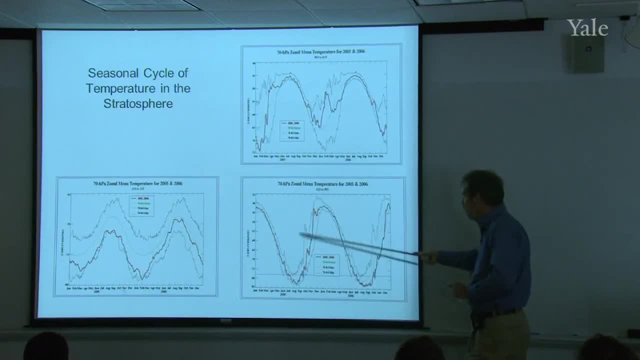 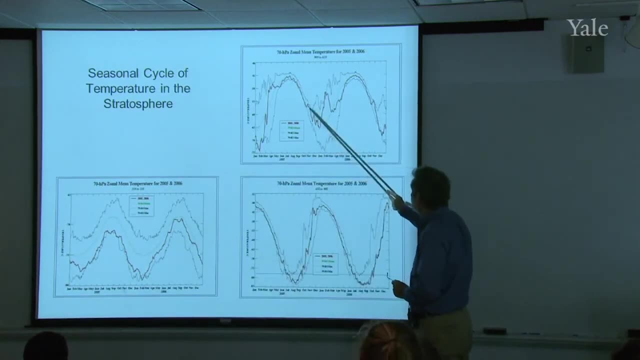 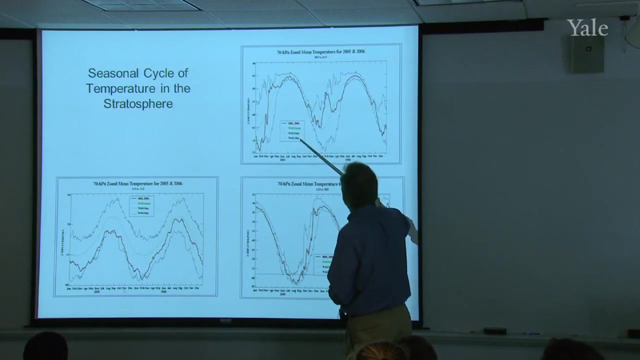 And this is 65 south to 90 south. So this is the south polar region. Now the temperatures in the northern hemisphere get down to minus 70 on occasion. These are at different altitudes I believe I'm having trouble reading those. 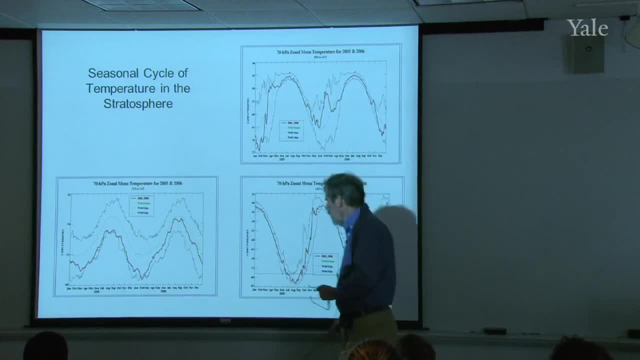 Okay. So they get down to about minus 70.. In the equatorial regions those temperatures get down to about minus 75. But here in the south pole they get down to minus 80 and even minus 85.. So, of all the places in the world's stratosphere, the southern hemisphere polar stratosphere that is, over Antarctica, has a wintertime temperature colder than any other place on the planet. That's one of the things that makes it special in regards to why the ozone hole forms there. Now, why would that be? 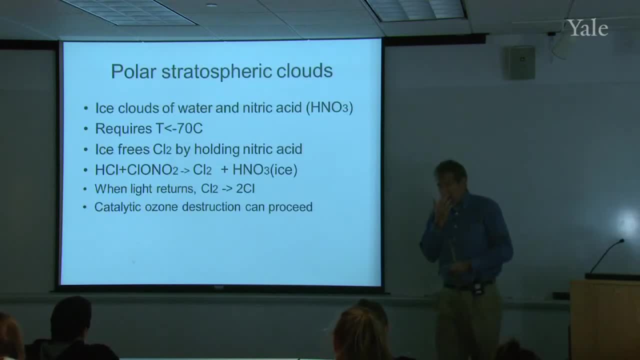 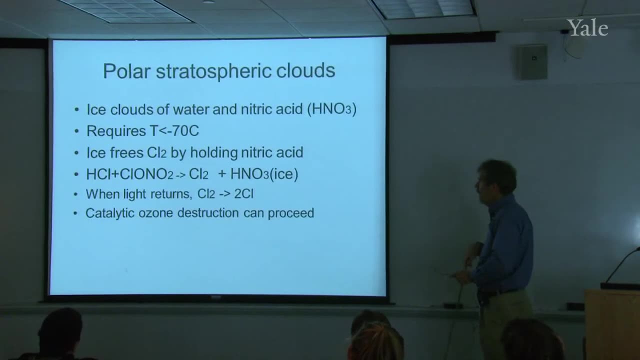 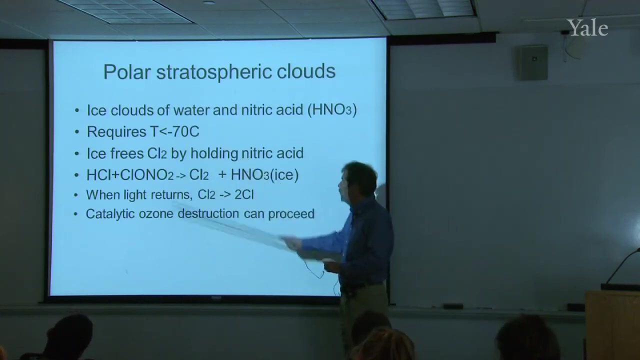 It has to do with the phenomena of polar stratospheric clouds- Abbreviation PSCs: polar stratospheric clouds. I haven't spoken about these in the course up to this present time, So this is new material. These are ice clouds that form up in the northern hemisphere. 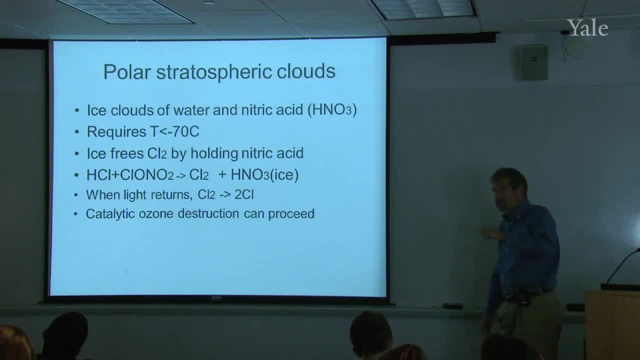 Normally we think clouds don't form in the stratosphere. It's pretty dry up there- but these clouds do. They are not entirely made of water. They're a mixture of water and nitric acid in these clouds And they require an extraordinarily cold. 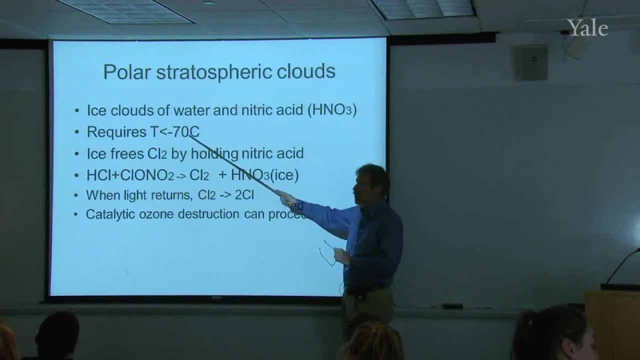 temperature in order to form Temperature is colder than minus 70 degrees Celsius. Some would say even colder than that. This is probably one of the most important things that we're talking about. This is why the Antarctic stratosphere is so special. 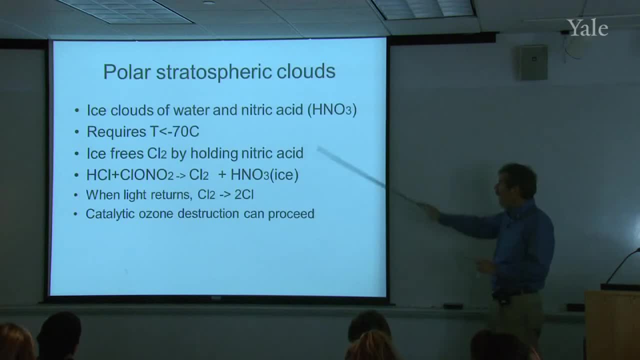 because its temperature gets cold enough in winter to allow these polar stratospheric clouds to occur, whereas other places around the globe, in the stratosphere, you don't get those clouds. What do they do, then? How do they influence ozone? Well, these ice clouds, these ice particles, freeze up. 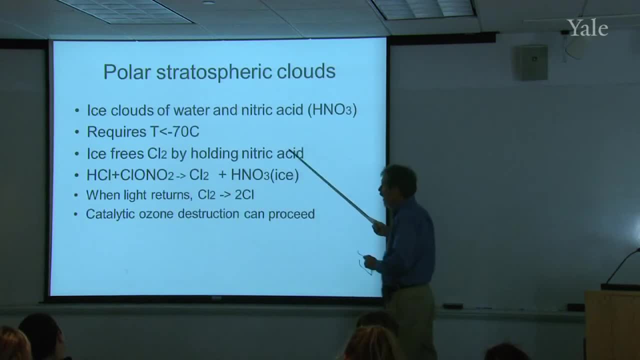 diatomic chlorine by holding the nitric acid in the ice itself. In other words, when it forms, it's storing HNO3, nitric acid. and here's the reaction. You start with HCl and ClONO2.. Reaction goes to Cl2 and the nitric acid, and then this is. 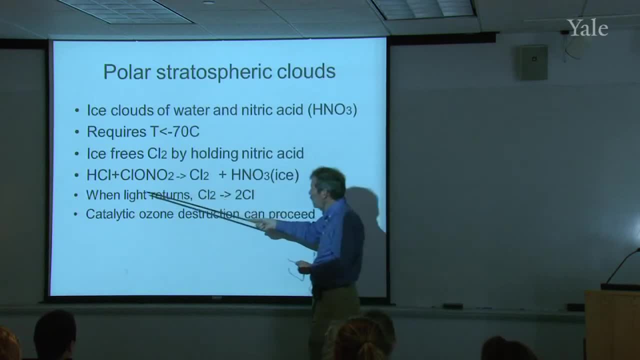 locked up in the ice. So what you've done, you had your chlorine locked up in the ice. It's locked up in HCl and in this compound. There's chlorines in both. Now you've put the nitric acid in the ice and you've freed up. 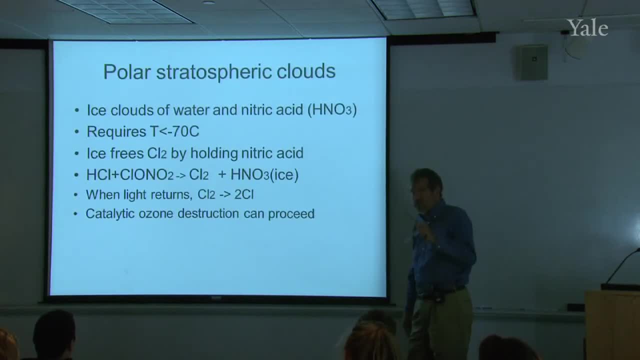 the chlorine diatomic molecule. There's only one step to go: When the light returns. remember that minimum of temperature occurred in perpetual darkness. At that season of the year, it's dark over Antarctica. There's no light, So you can get the ice forming. you can get the Cl already in. 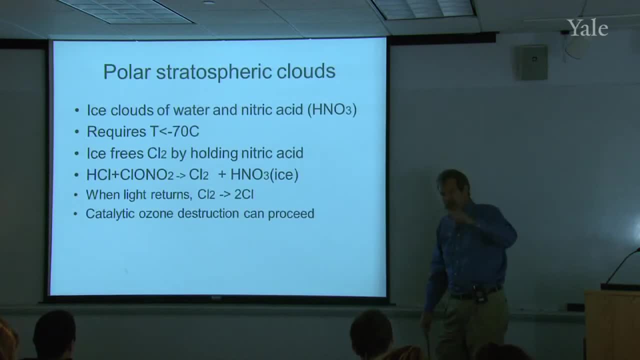 ready to go, but it's in the diatomic form. Then the light comes back. southern hemisphere spring. the light comes back. You can dissociate the Cl2 to form two Cl molecules and then go back a few slides to that catalytic reaction and it. 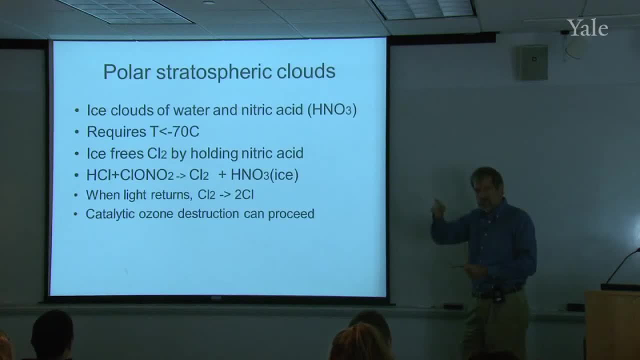 starts, it starts to destroy ozone. So you get that. So the ice frees up the chlorine. it then dissociates when light returns And the catalytic destruction of ozone begins to take place and the ozone hole forms. That's why it occurs where it does and when it does. 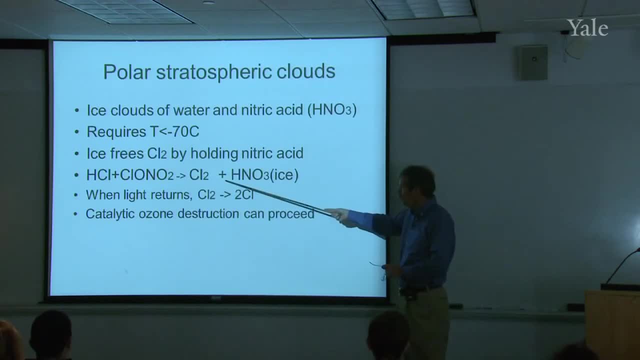 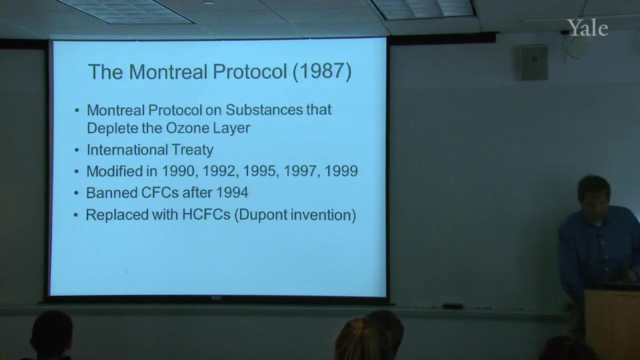 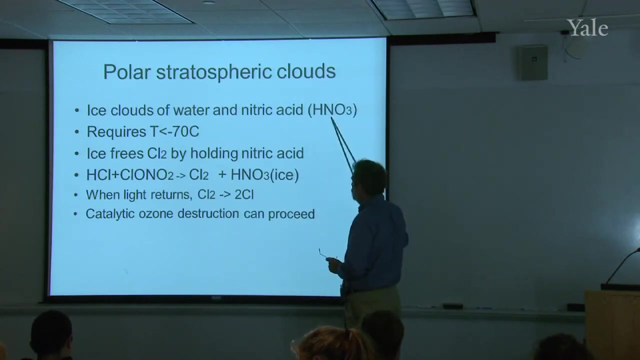 Because of that necessary condition for cold, And then the ozone hole forms just after the light returns to that region. Any questions on that? Yes, I don't know. That's the way the chlorine is stored most of the time in the stratosphere is in these two molecules. 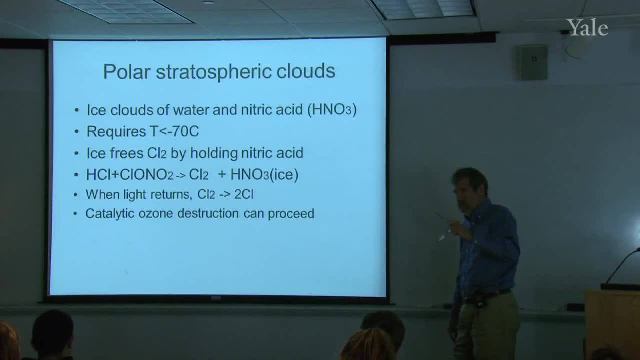 After the CFCs break down, the chlorine is transferred into these two forms and just hangs around. Then the PSCs form And that sucks off the Nitric acid and the Cl is released. So this is the storage form of the chlorine during most of 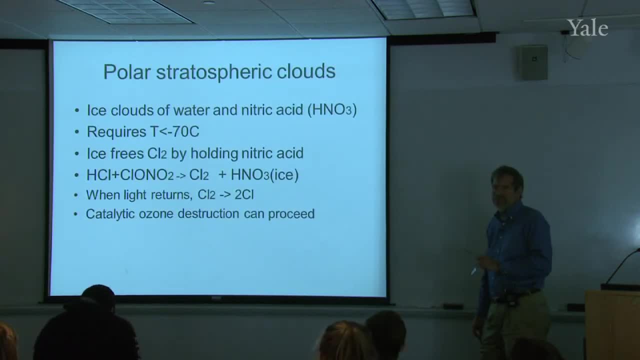 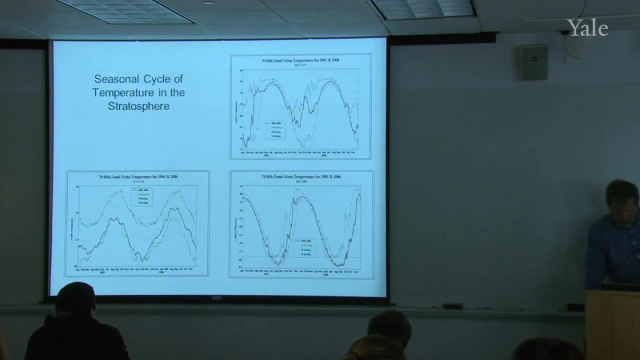 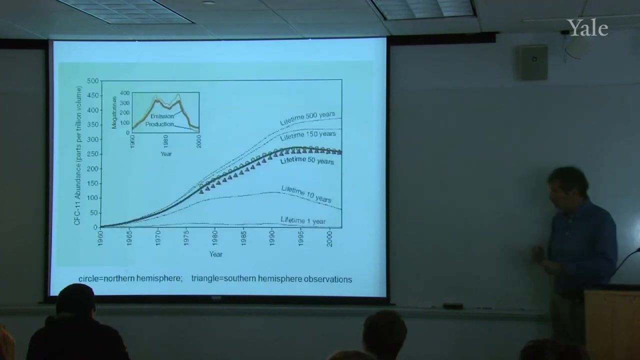 the year in the stratosphere, Not naturally, Remember this. no, this was CFCs and not chlorine, And that's a critical difference. But let me just go back to that. There were no CFCs in the atmosphere. 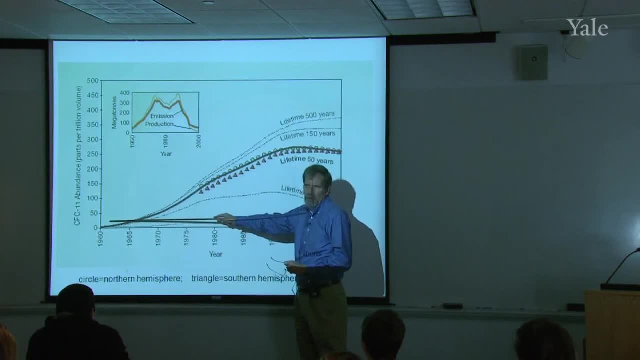 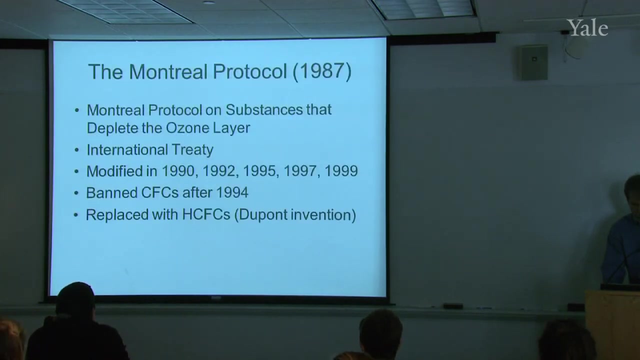 There probably was a little bit of chlorine, but only a very small amount, But now we're putting it in through this CFC source. So that's not a complete answer, but that's the best I can do. So I think this is the last one. 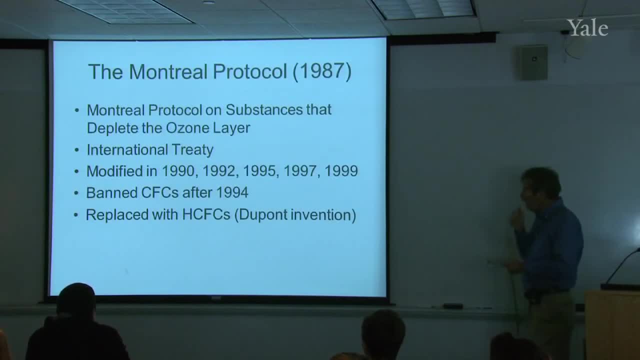 So the Montreal Protocol. the full name of it is Montreal Protocol on Substances That Deplete the Ozone Layer. It's an international treaty and of course it was first signed in Montreal. it's got the name. Since then it's been modified several times. Certain forms of substances have been added to the banned list, others have been allowed, so it's been modified a few times. Generally, what it did is, by the time we came to 1994, it had banned pretty much all emissions of CFCs into the. 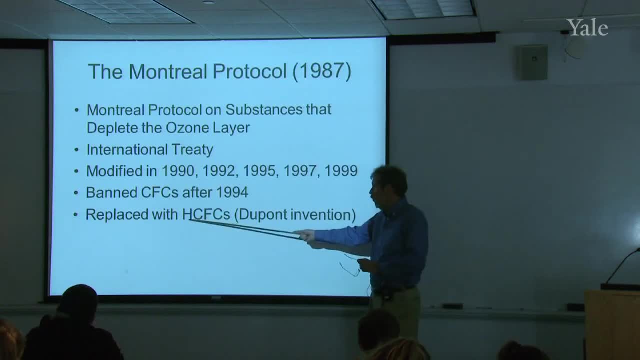 atmosphere. It largely replaced them with the H-CFC, which can also be used as a refrigerant, but has a much shorter lifetime and will not cause the chlorine to build up in the atmosphere. It may have some other problems. It may be a greenhouse gas, but it doesn't have the 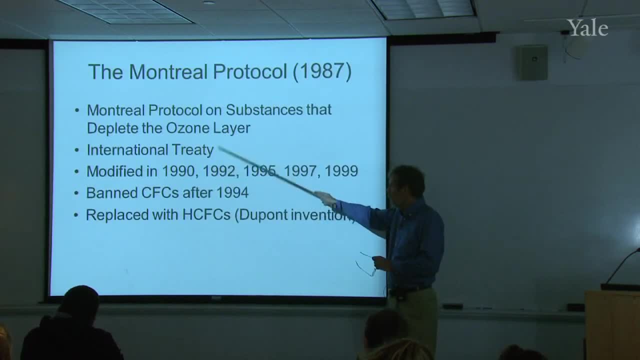 problem of putting permanently chlorine into the atmosphere the way that they do Now, one of the reasons why this treaty was signed- because, as you could expect, the refrigerant industry vigorously opposed this was that, about the time it was signed, DuPont, which was this large chemical company, and the 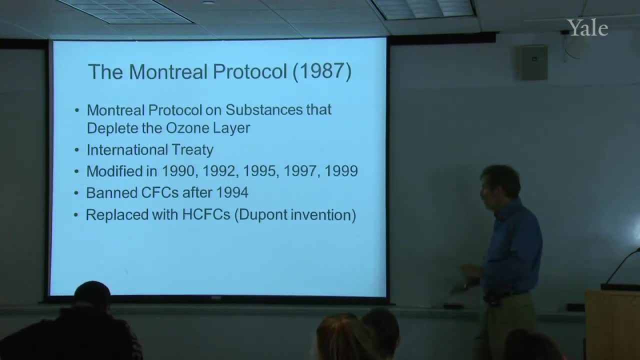 world's largest producer of CFCs, discovered a replacement for it And they realized that they would not lose their business because they had to, Because they had a replacement ready to go, and they might even be able to make more money by doing this.